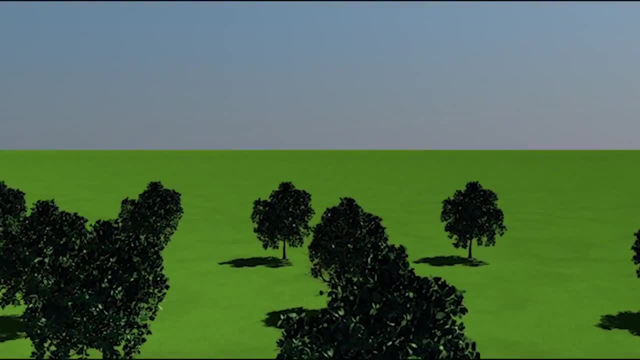 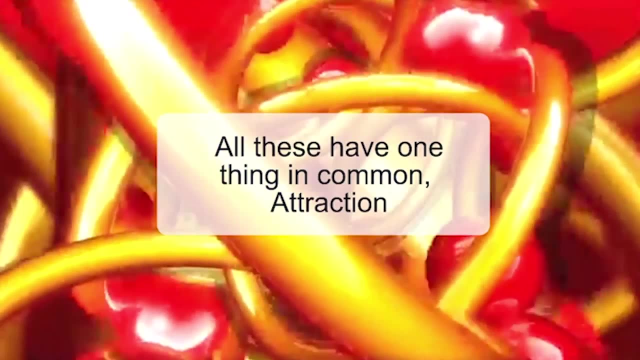 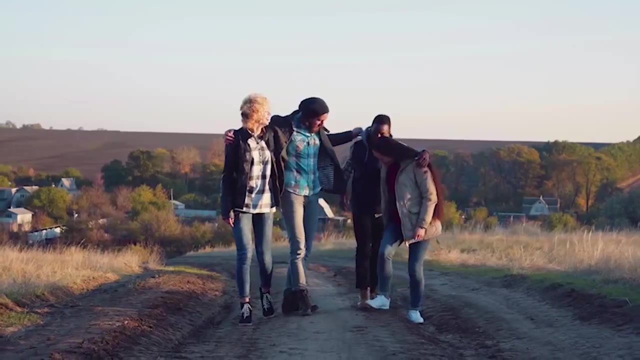 or why we often see objects as fruits always fall towards the ground. All these have one thing in common: attraction. Without attraction, the planets will lose their stability and collapse into the sun. There will be no desire for, or attraction between a man and a woman. 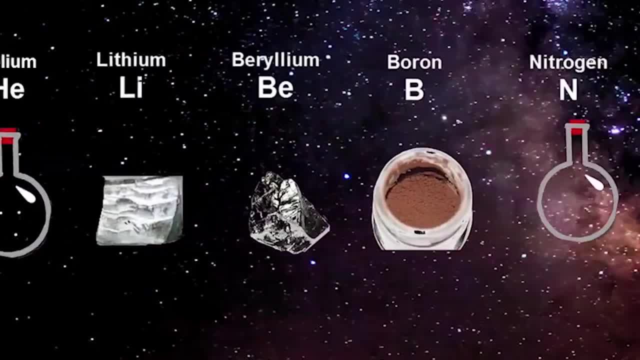 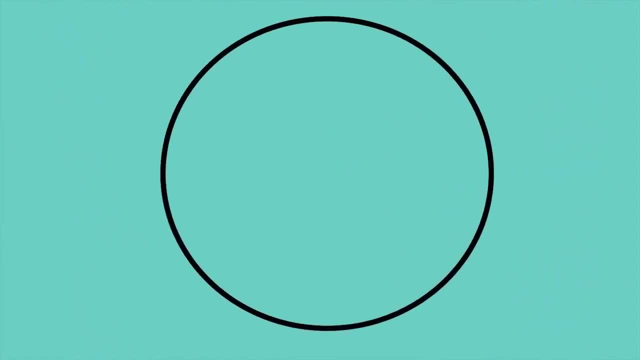 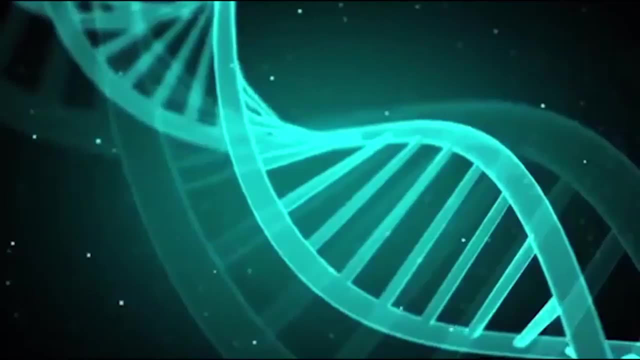 Neither will fruits always fall to the ground. Similarly, all substances in our universe, like water for instance, are made up of tiny particles called atoms, molecules and ions that always attract each other. Our DNA, the source code of life, also contains several molecules attracting each other. 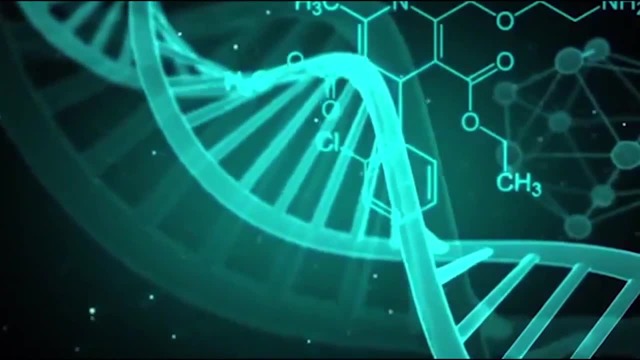 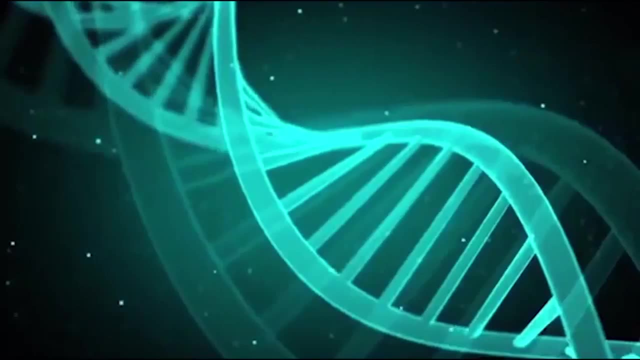 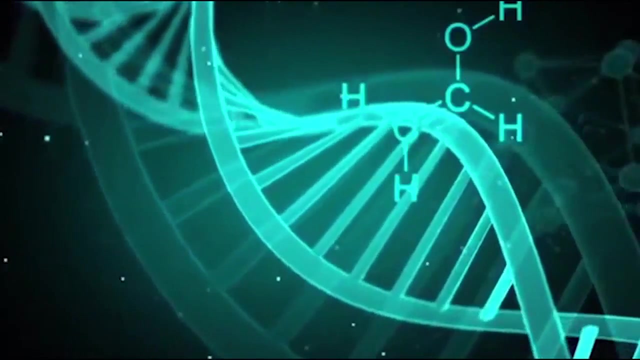 Implained that the very basis of life is built on the force of attraction between billions and trillions of atoms, molecules and ions found within and around us. The attraction or force of attraction that occurs between these individual atoms, molecules and ions is what we call chemical bonding. 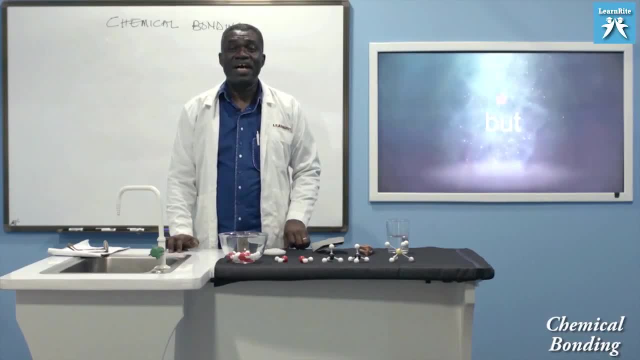 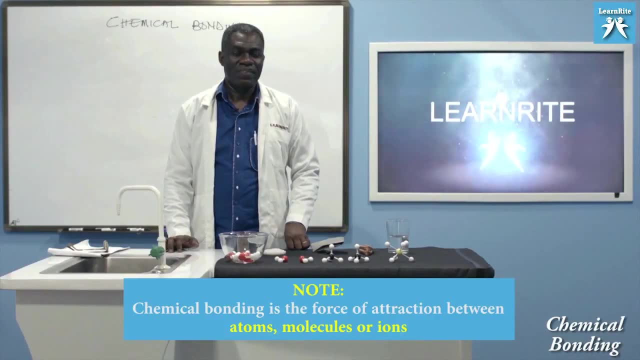 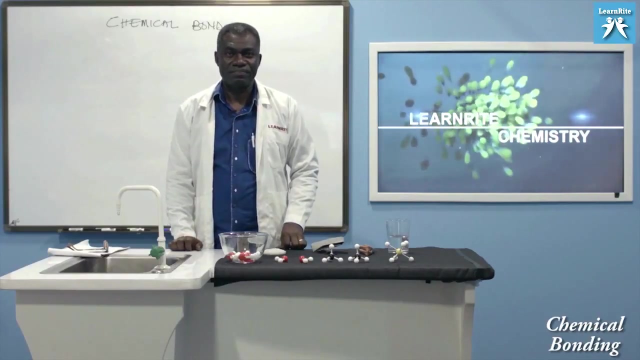 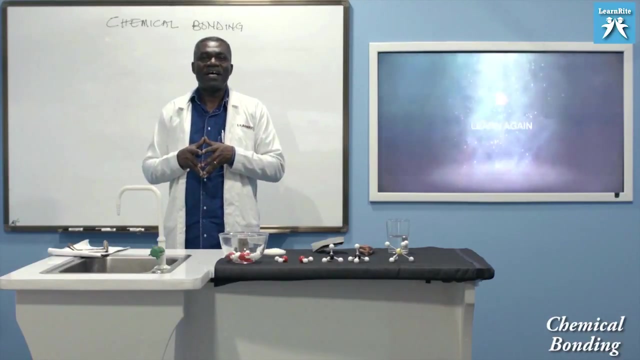 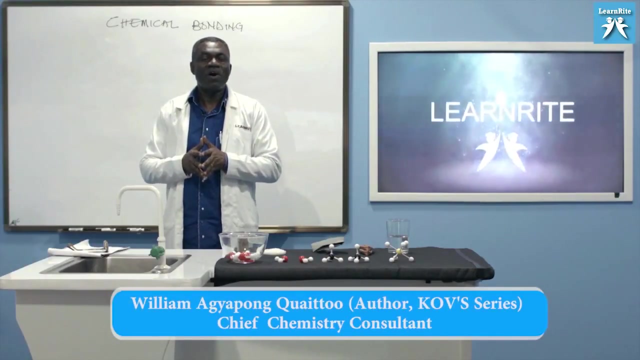 In short, chemical bonding may be defined as any force of attraction between atoms, molecules or atoms. In chemical bonding we have two main types. We have two main types of chemical bonding: One between atoms that make up maybe a molecule, which often is referred to as primary bond. 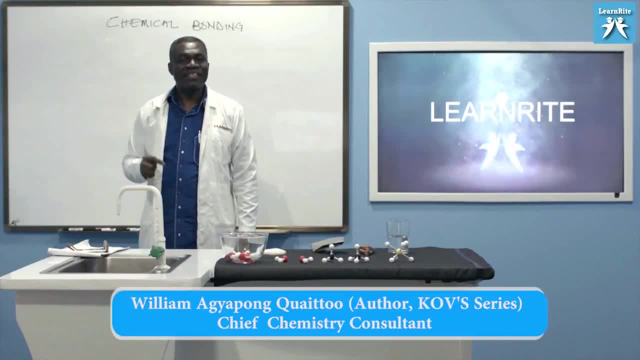 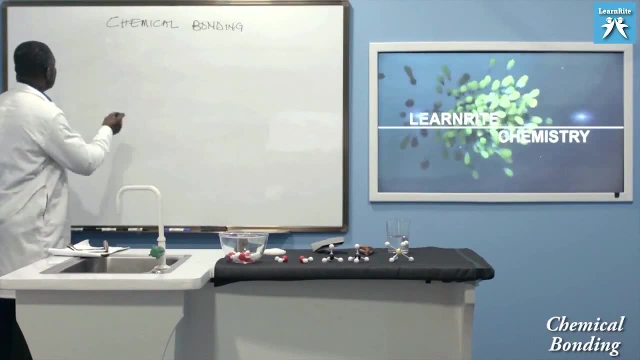 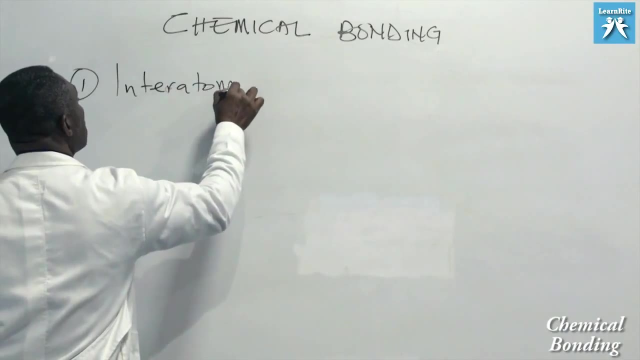 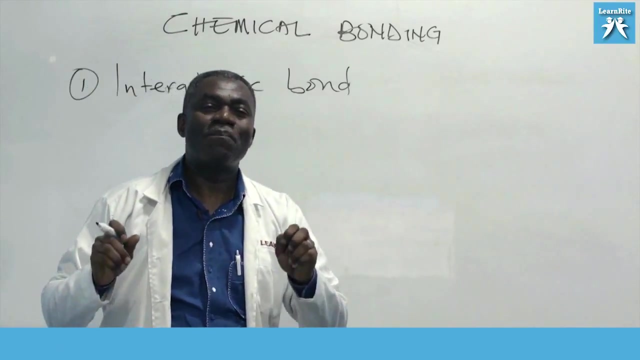 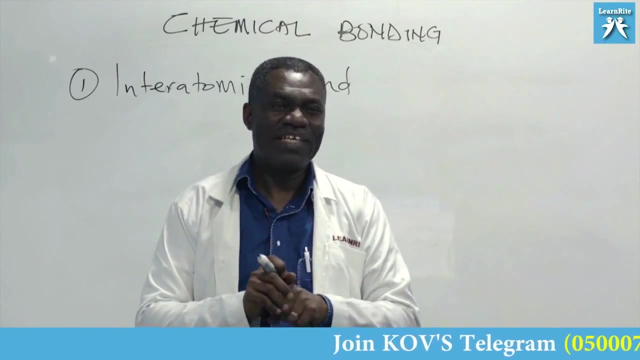 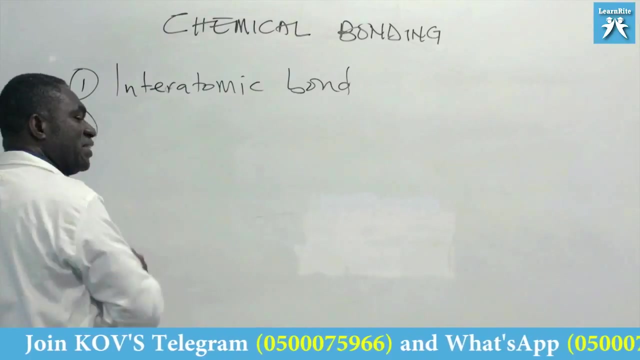 but specifically called inter-atomic bonding. Inter-atomic bonding- The word inter-atomic simply means that the bond or the force of attraction is occurring between two or more atoms In one molecule. In one molecule We also have a second type of bonds. 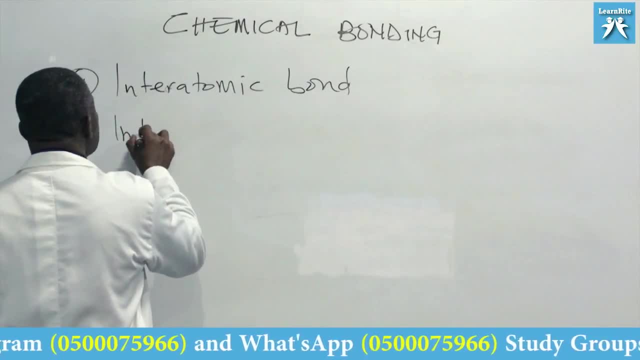 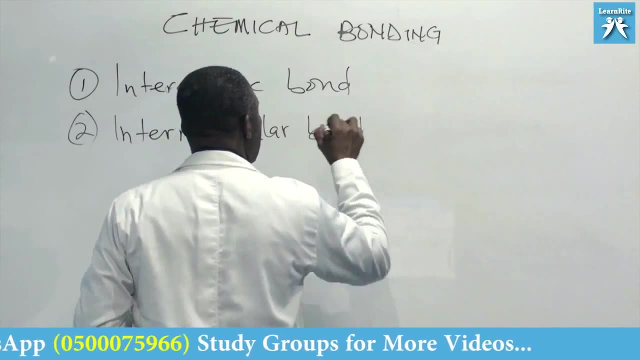 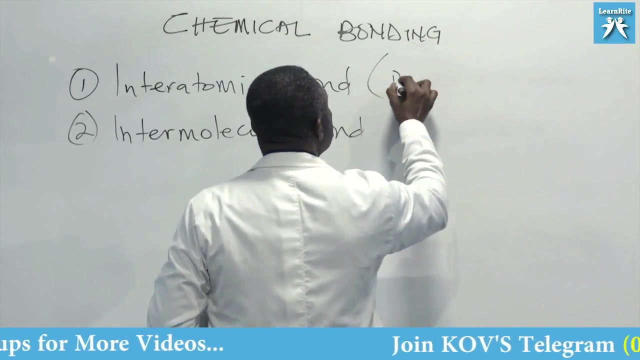 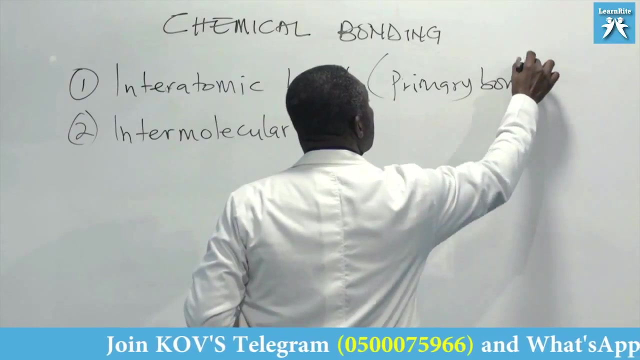 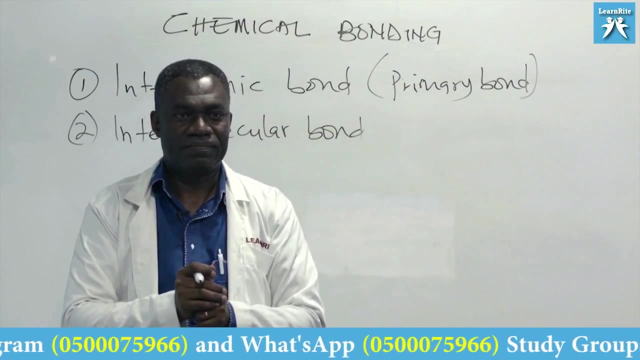 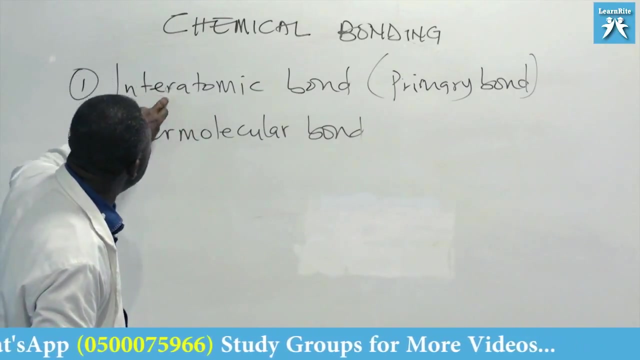 called intermolecular. The inter-atomic bond, which sometimes is referred to as primary bond, may occur between only one mole or one molecule of a substance, The intermolecular. look at the words. Let me explain. This is inter-atomic. It means that between: 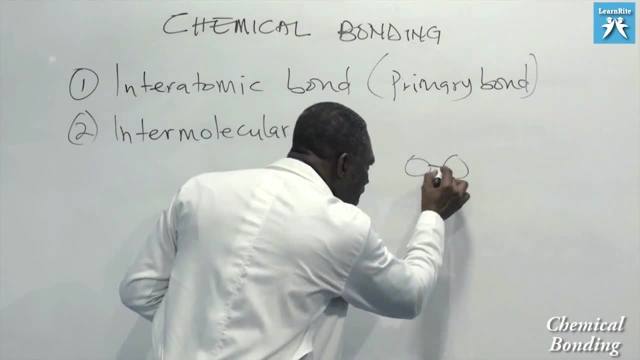 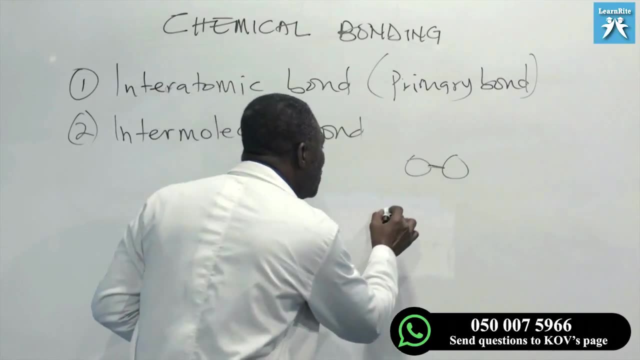 one atom and another atom, then there's a bond here. Okay, The intermolecular means that we are going to talk about intermolecular, So there's a molecule, so that if we have this and that as a molecule, then we have another one there. 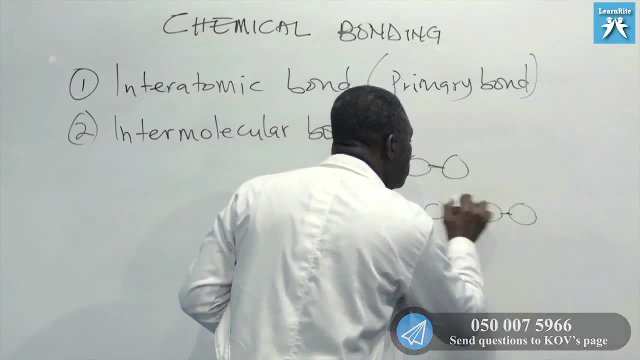 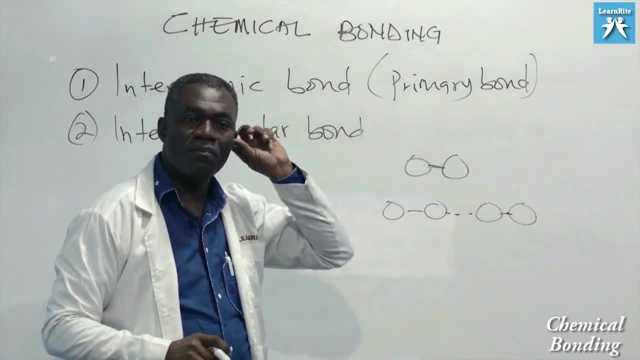 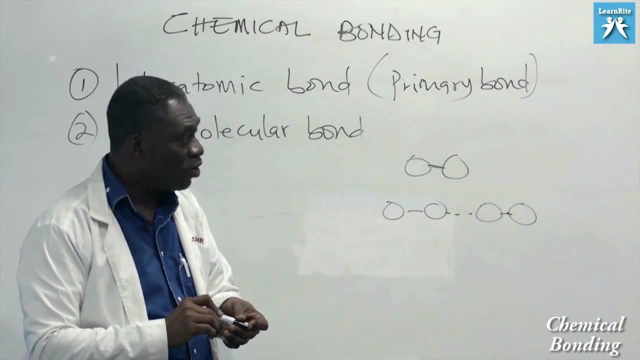 There could be another bond between them. So the bond between this one molecule and that one molecule is what we call the intermolecular bond, Whereas the first bond between this atom and that atom is called the inter-atomic bond. So the first one. 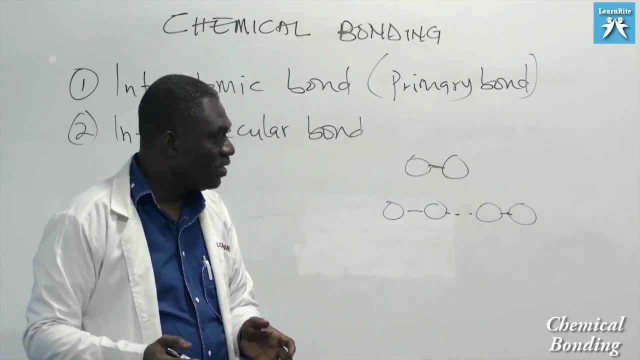 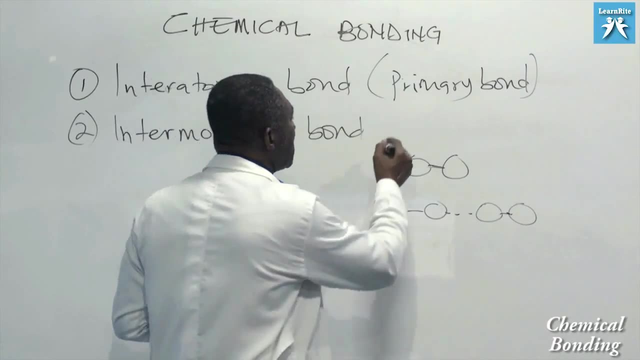 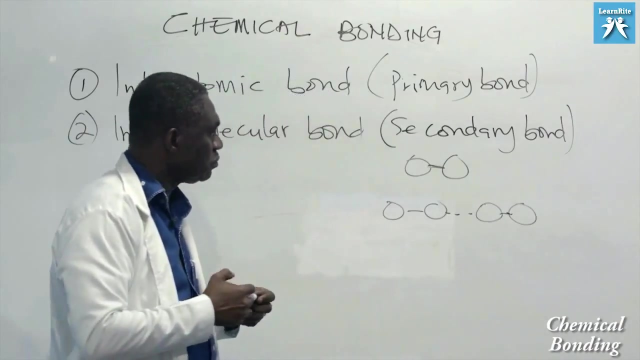 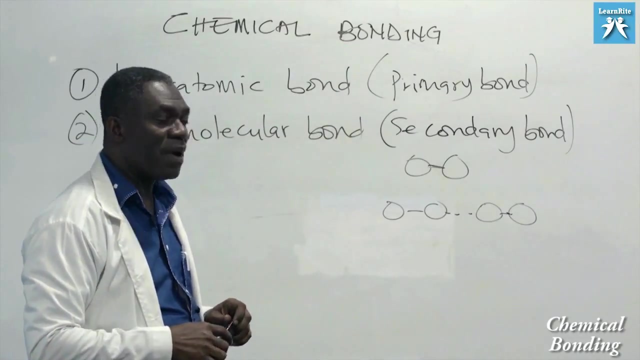 is between atoms in a molecule, and the second one, which is the intermolecular bond. is the intermolecular bond? It's between a number of molecules, which is sometimes referred to as secondary bond. We have three major types of the primary bonds or the inter-atomic bonds. 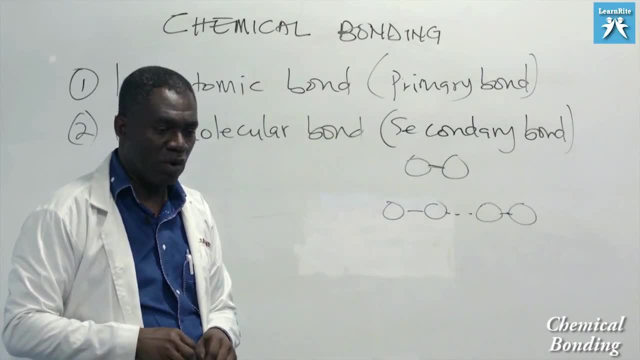 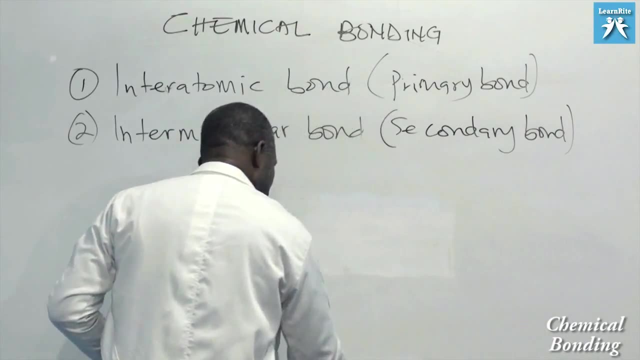 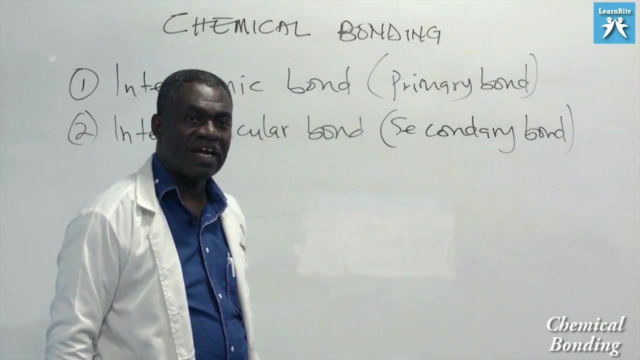 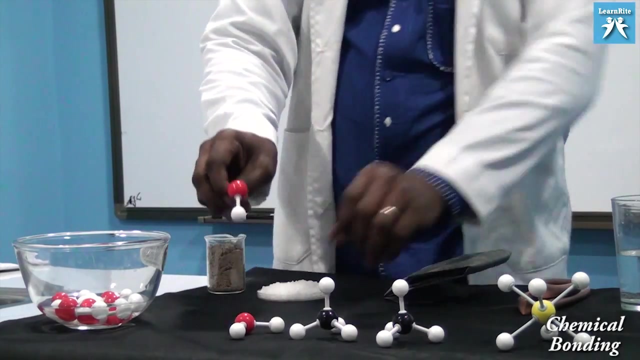 and we have about four types of the secondary bonds. Before I go to explain that, I want to come to the table and illustrate the types of bonds that I've mentioned. Now let's take this thing that I'm holding as an illustration. 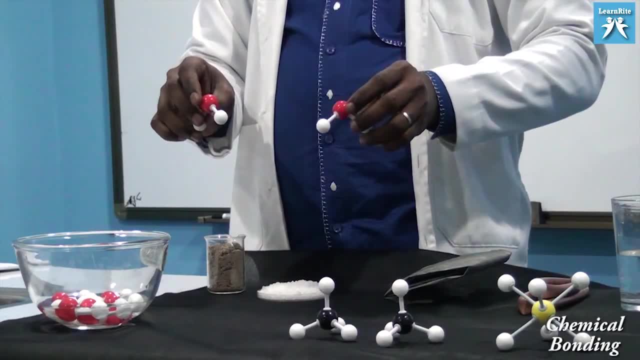 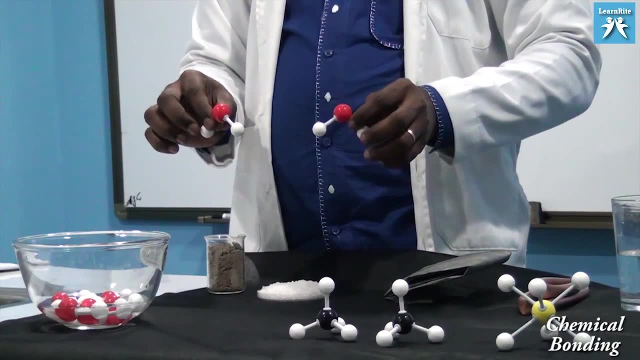 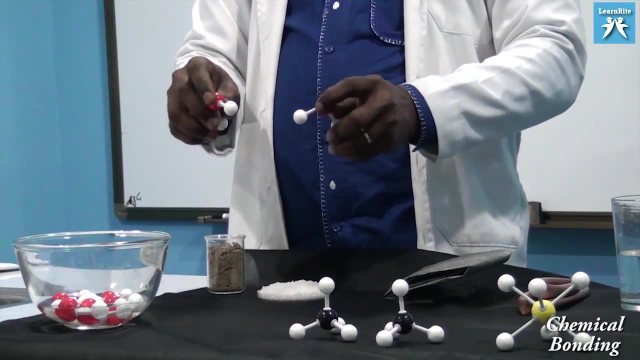 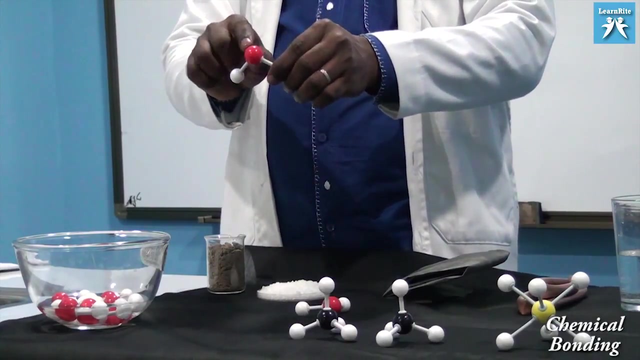 This molecule here is a magnified water molecule In chemistry. very soon you'll grow in chemistry and I'll explain to you that this structure that I'm holding here represents water molecule, where the red ball here represents the oxygen and then these two white balls. 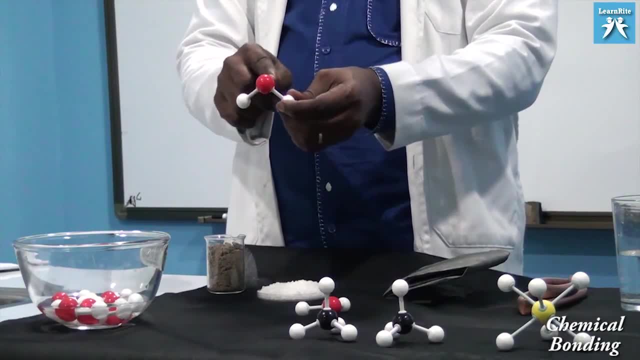 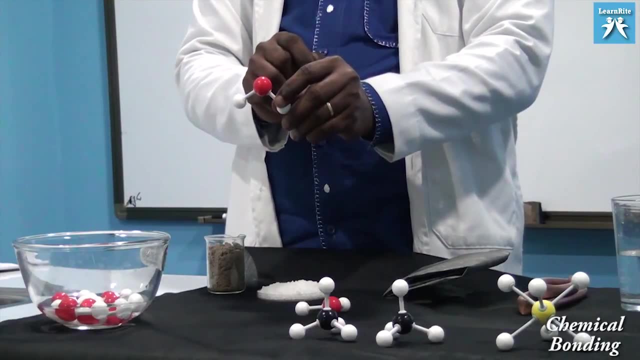 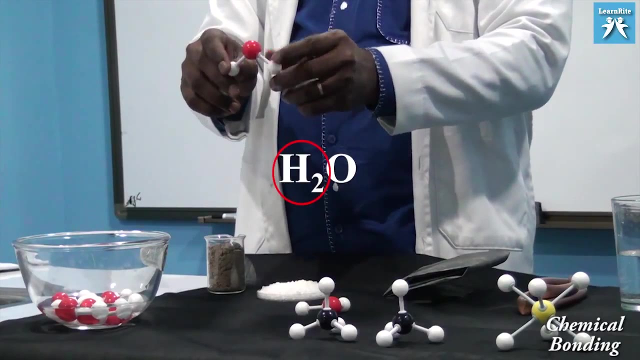 represent my hydrogen atoms. They are bonded like this. So oxygen is bonded to hydrogen here and this oxygen is also bonded to another hydrogen here. Remember that the formula for water is H2O. Okay, two hydrogen atoms and then one oxygen atom. 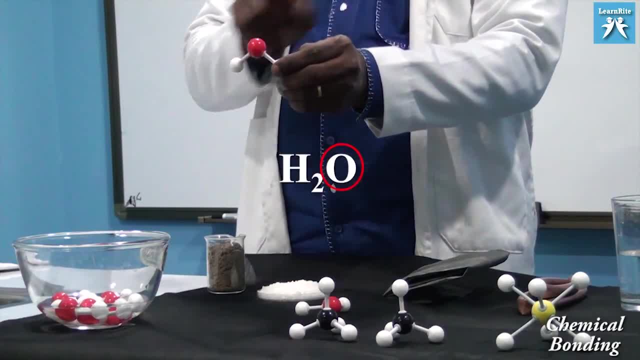 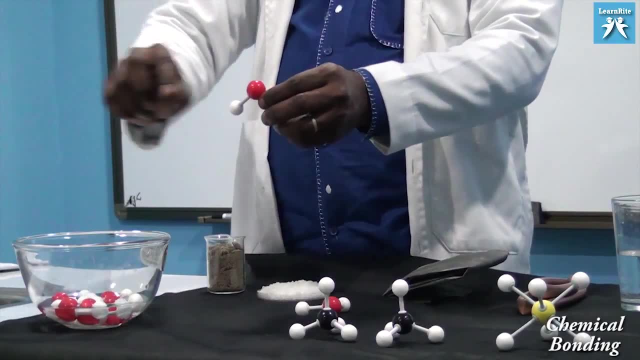 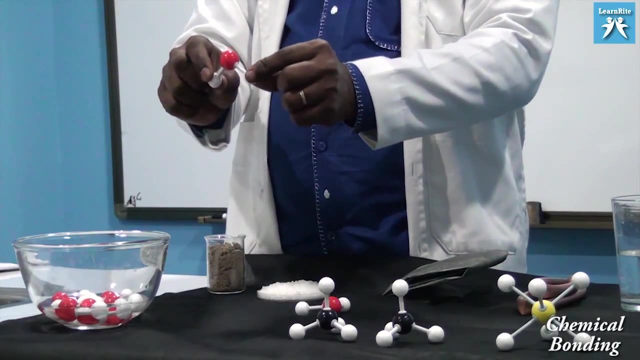 Two hydrogen atoms, which are represented by the white balls, and one oxygen atom, represented by the red ball. Now, why are they not, maybe horizontal? Why is the bond here not horizontal, but in an angular shape? That you will know when you grow, But that is. 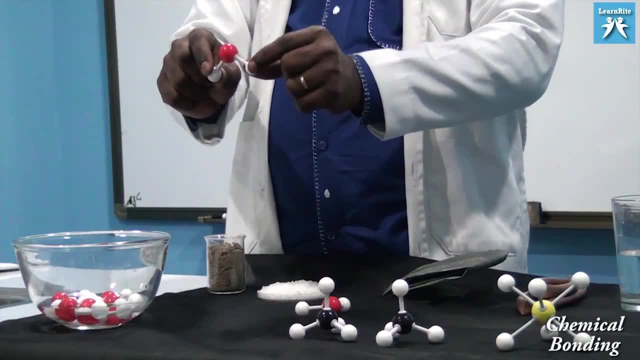 the shape of a water molecule. But that is the shape of a water molecule. But that is the shape of a water molecule. It is not straight, It is not horizontal, It is bent at an angle. We'll explain it when we grow in bonding. 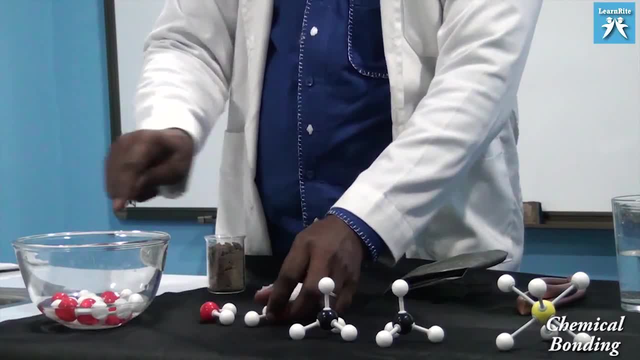 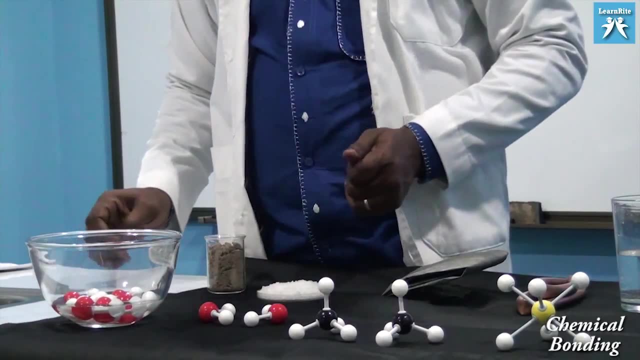 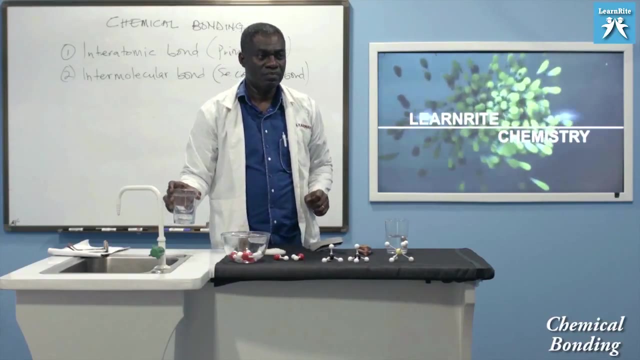 Okay Now. so if you have water molecules, if I take this water here- there's water in here- or I take water that I'm pouring here, you see it running through. You see it running through straight into this water molecule. 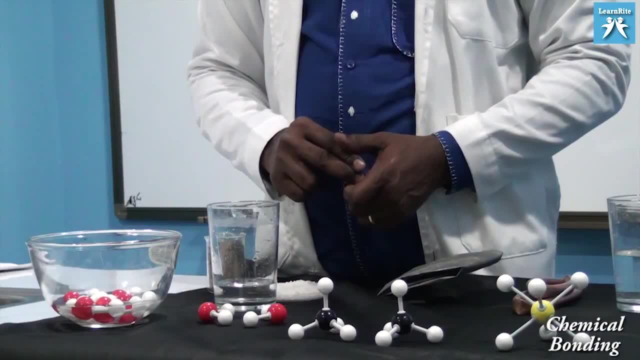 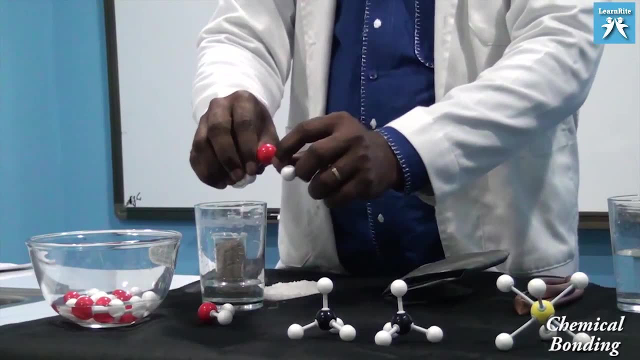 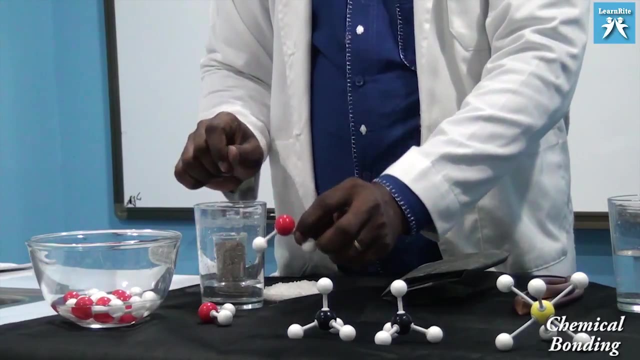 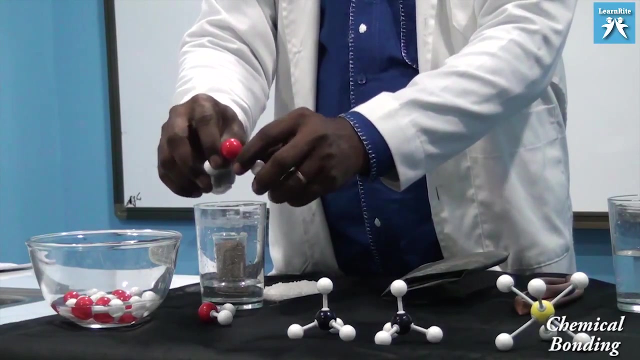 Into the beaker. We are not seeing the water molecules, as I showed to you In the water We are not seeing them. Okay, But this water here and the other water molecule here suggest that we have several millions or trillions of these water molecules in there. 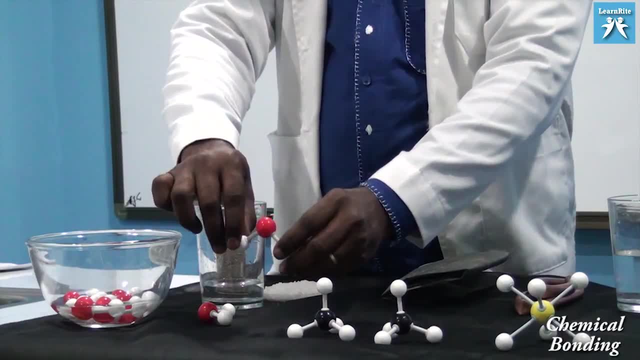 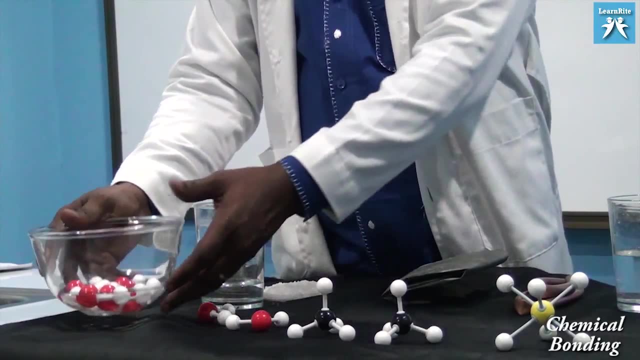 These water molecules in there. So it is just one molecule. that is the studying. So it is just one molecule, that is the studying. you pick a magnifier, you see the shape to be like this. so, like in this container, i have water in. 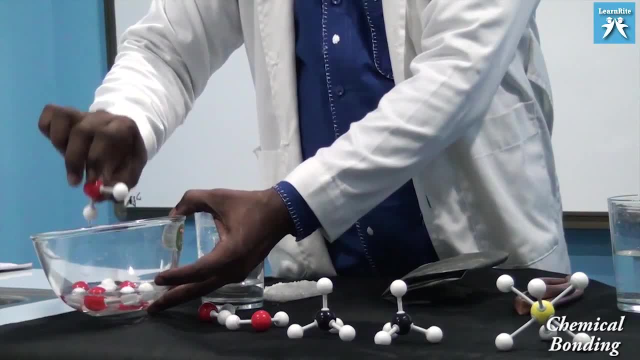 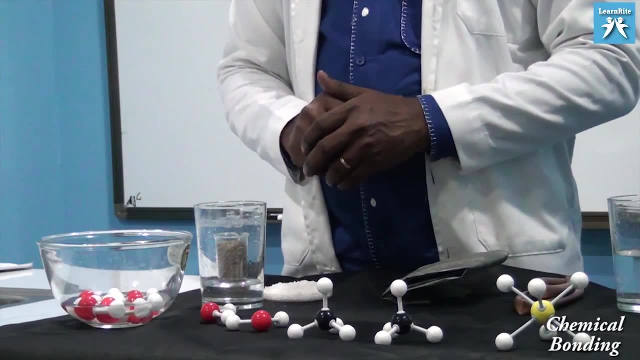 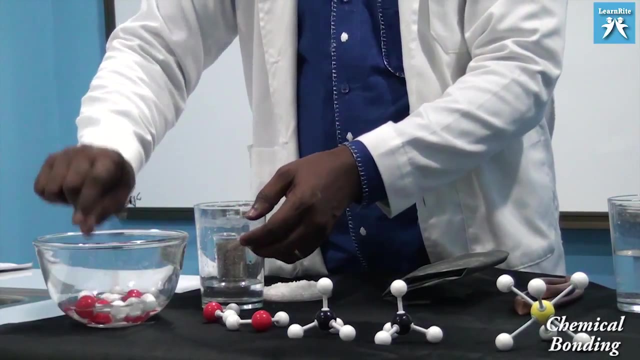 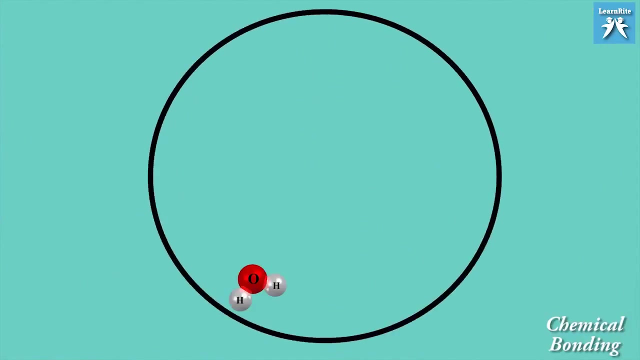 there and i put in the molecules of the water in it. what i'm trying to illustrate here is that in the water molecules here, that is the volume of water within it- we have several of this in there and how they bonded if you use a magnifier to magnify any volume of water. 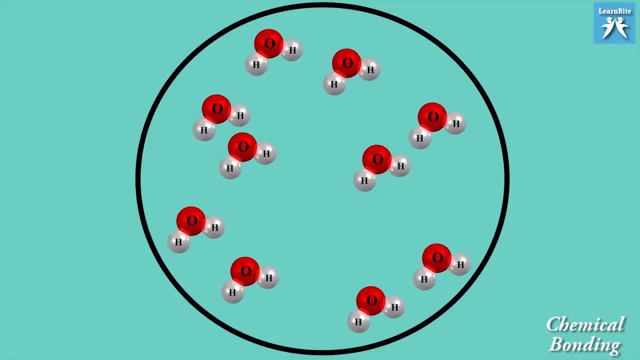 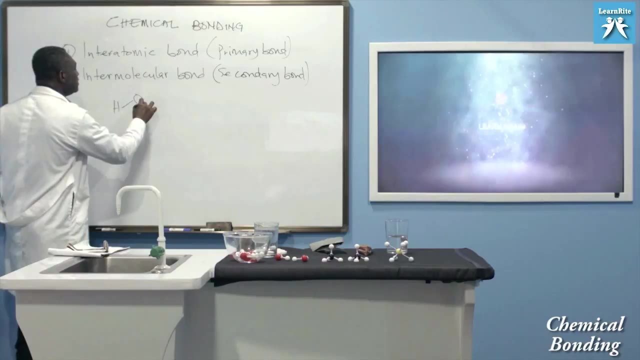 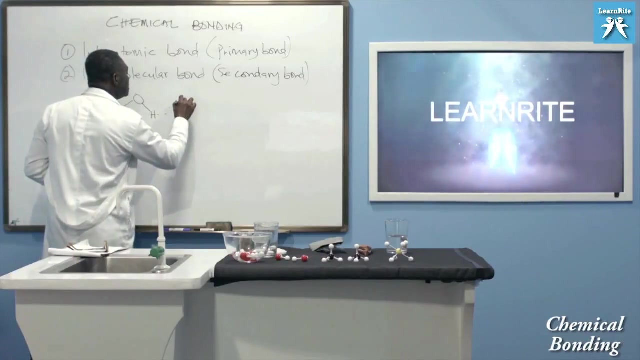 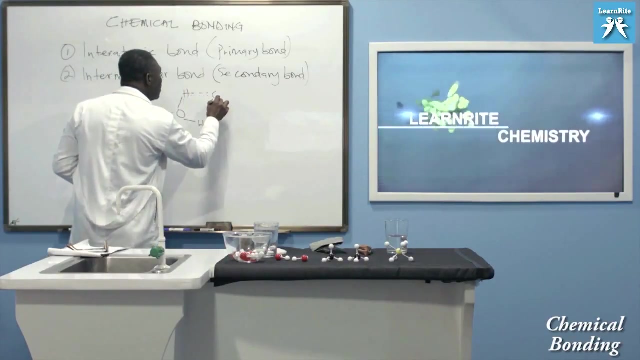 that is how you are going to see the molecules, or the particles of the water molecules, arrange. you see them as you see them, as hydrogen bonded to oxygen, and then another hydrogen- okay, and then here this could also be bonded to oxygen- and then hydrogen hydrogen, and then it will continue: oxygen, hydrogen, hydrogen. 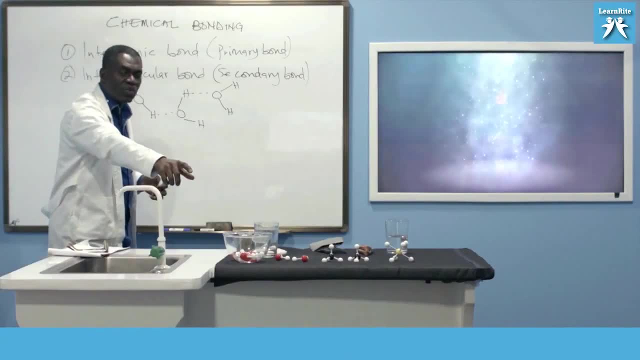 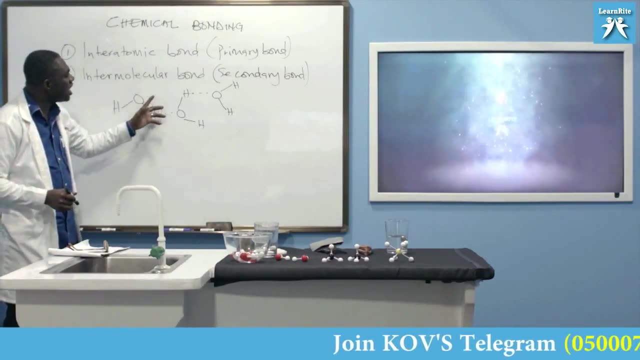 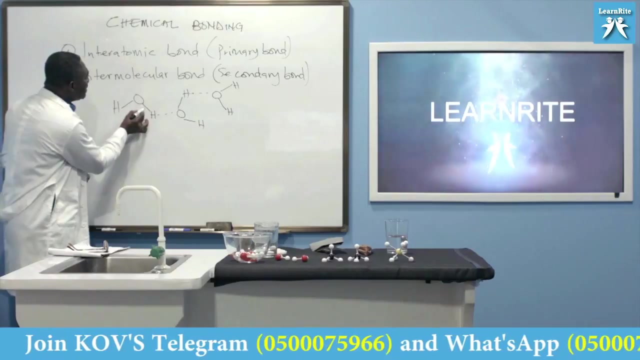 so they come together for us to be able to see the water as we see it in there, bigger, all continuing. now, why is it that i'm joining these atoms with different types of the different types of lines? it's telling me that this is a primary bond, an interatomic. 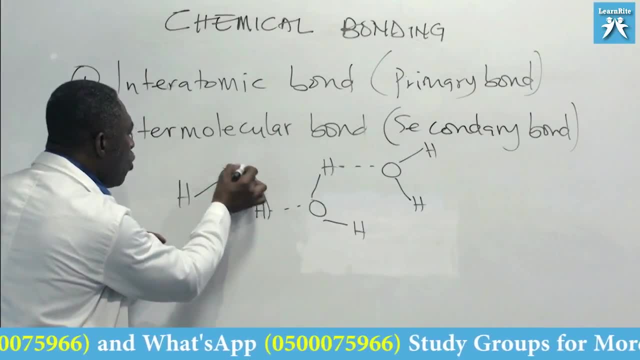 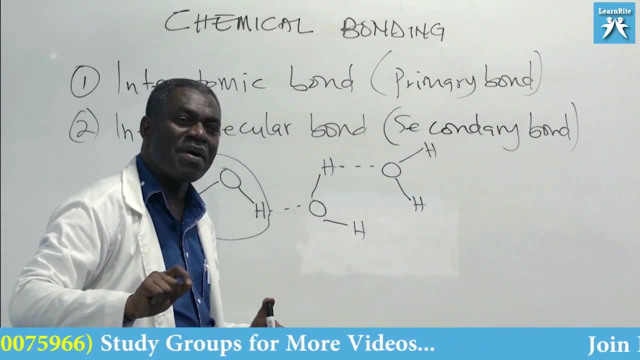 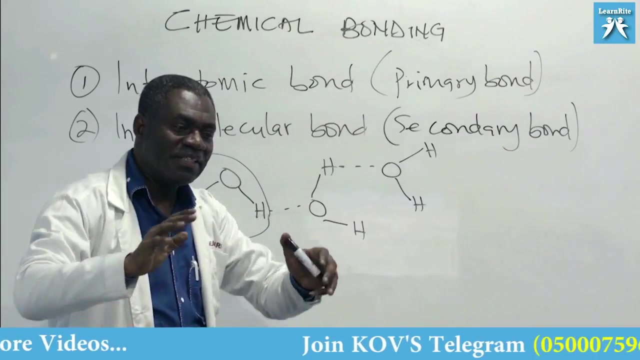 oxygen hydrogen. oxygen hydrogen for one mole or one molecule of the water. but because when i begin to pour the water they don't come out one by one like a drop and then another drop will come, it is telling me that the volume of the water is also. i mean the molecules within the total volume of the water are also bonded. 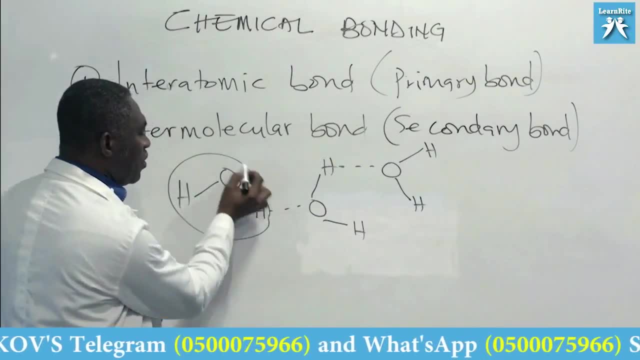 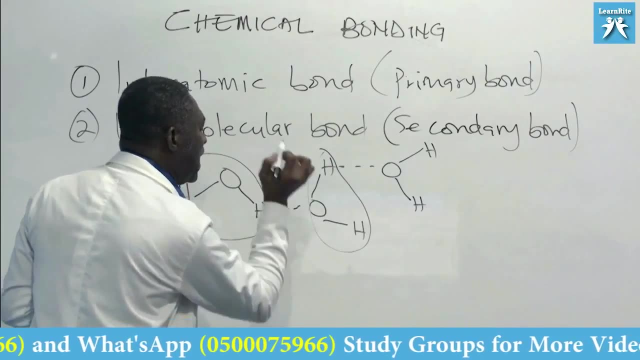 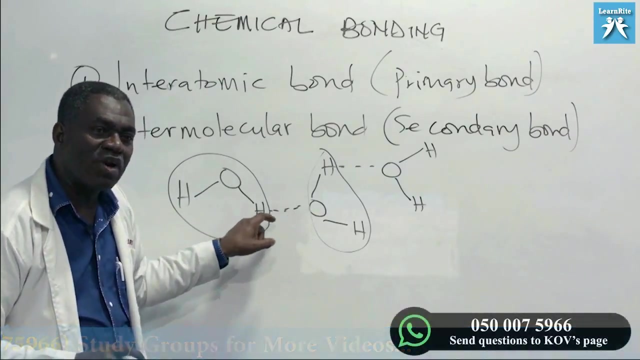 together, and so it means that this mole of water or this one mole or one molecule of water is bonded to this one mole by the dotted lines. so, in short, i'm separating the interatomic bonds from the intermolecular bonds with the straight line and then the dotted line. they are both. 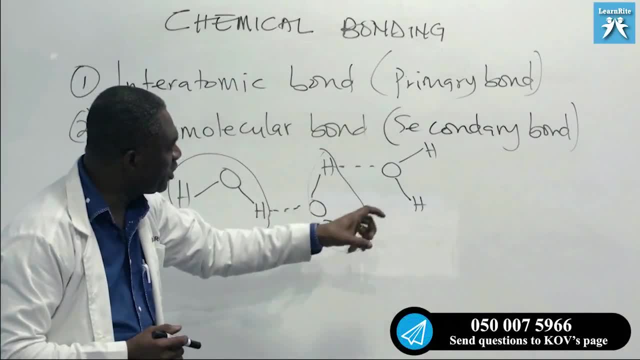 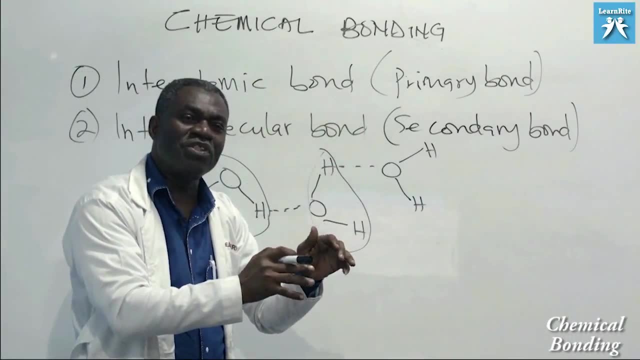 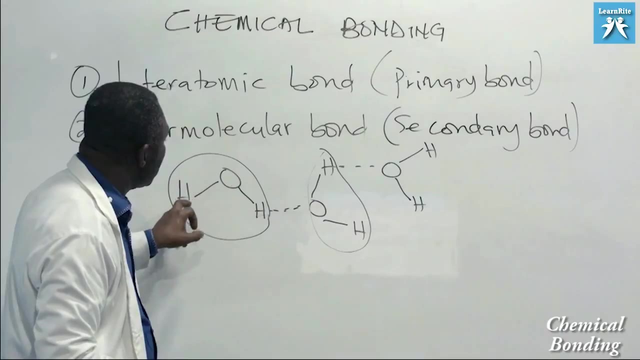 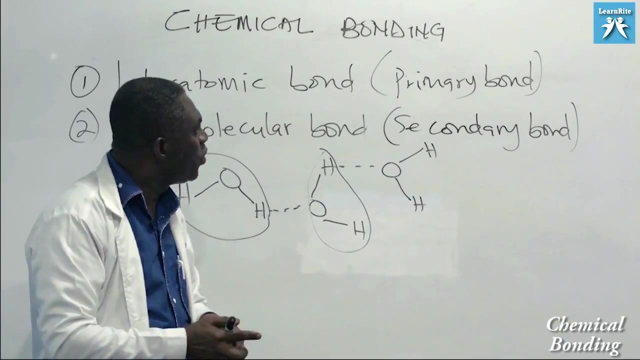 representing bonds, and in this illustration the dotted line is presenting my intermolecular bond, a bond between one molecule of water, another molecule of water and another molecule of water, but within that molecule of water the atoms are also bonded together. so these are the two major types of bonds we have: interatomic, which some people also call intramolecular, if you say this. 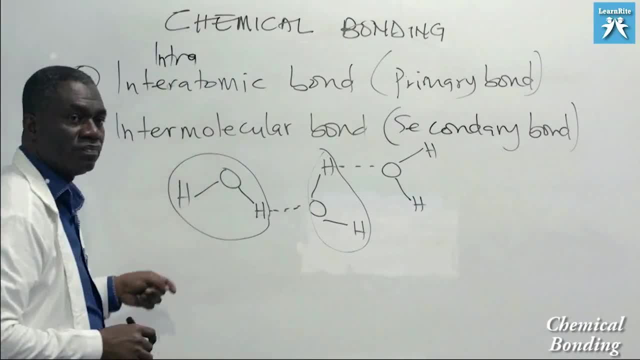 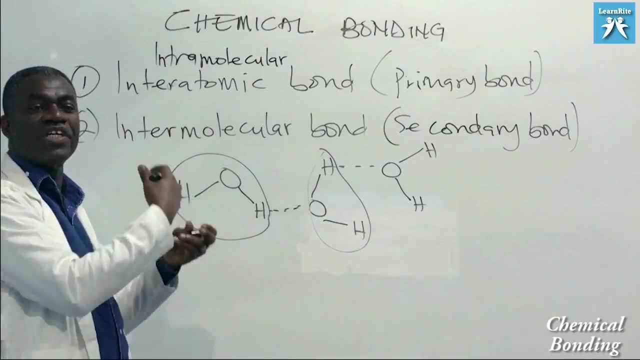 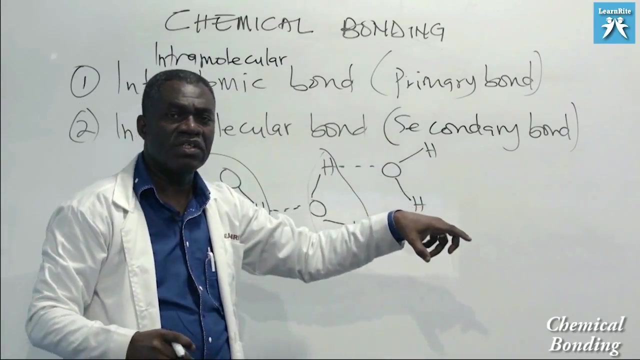 if you say intra, it means intramolecular. if you say intra, it means intramolecular. if you say intra, it means within. you can say intramolecular, that is, within one molecule. the bonds there is the same as intra-molecular, the same as inter-atomic, and that's the first type of bond to form one molecule. 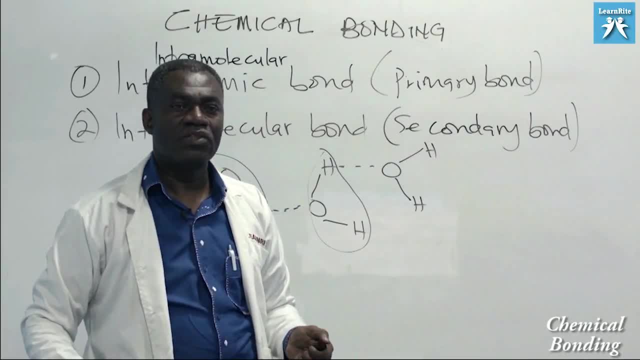 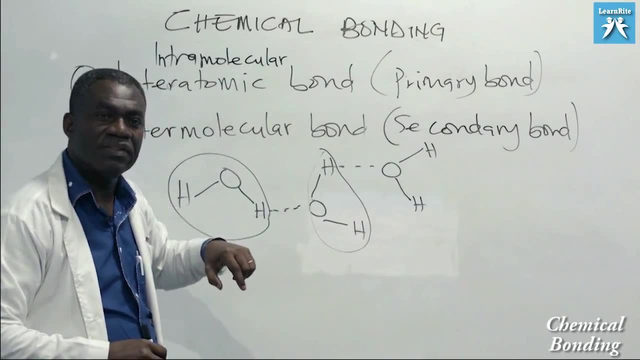 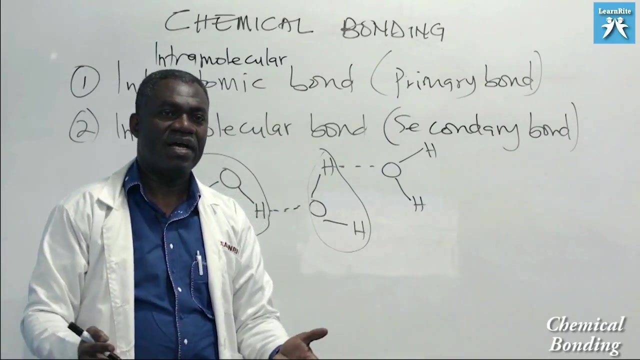 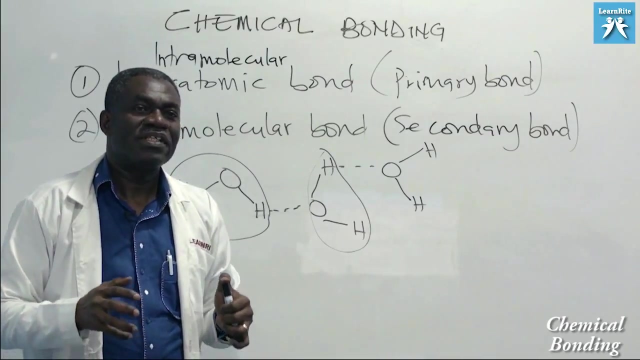 before. the molecules can also be bonded to each other to form the entire substance that we are referring to here. i'm using water as the substance within the water substance. we have water molecules that form that water as a substance and within that substance we are seeing two types of bonds: the bonds that hold the atoms of each molecule together. that is the primary bond. 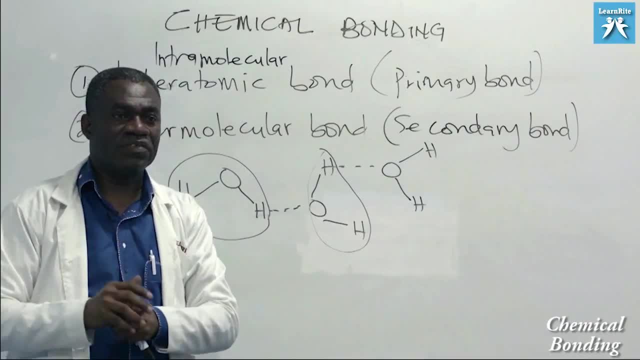 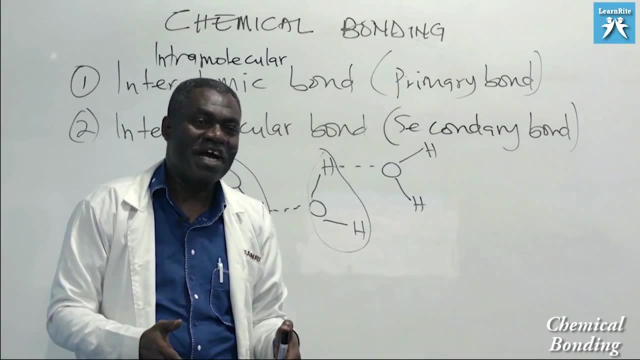 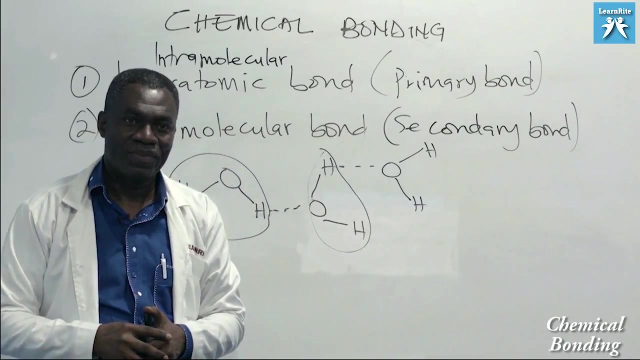 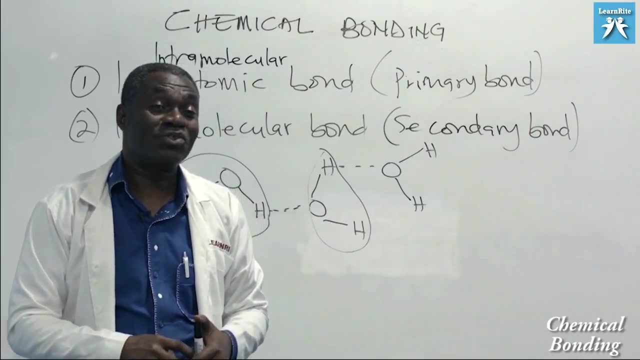 the bonds that holds each of the molecules to themselves. simply put the attraction between members of a family, and then the attraction between the families, and then the attraction between a family and another family. okay, and what do you think the strength of these bones will be? the bond between a sister and a brother and a mother, compared to the bond between one family? 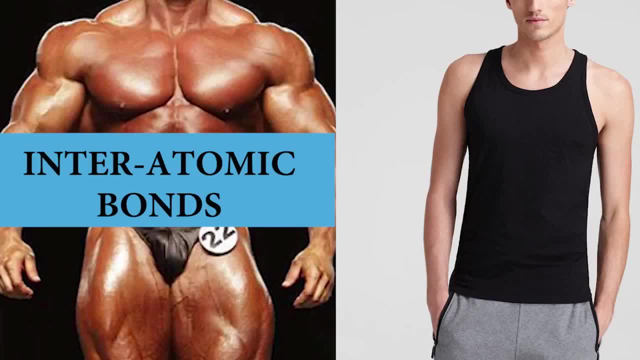 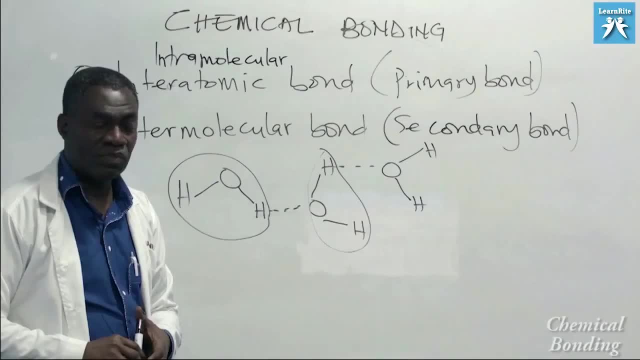 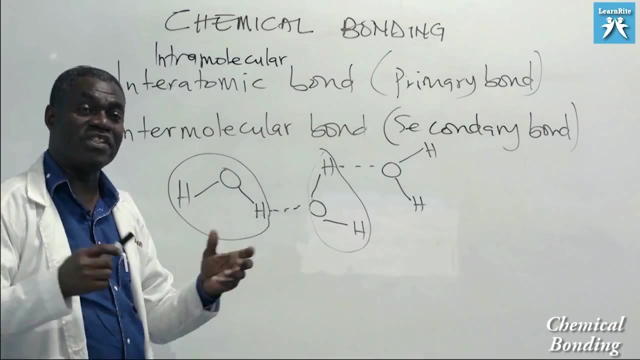 and another family. simply put, inter-atomic bonds are mostly stronger than inter-molecular bonds, because several reasons work out for that. we'll be doing all these in series in our next videos and we see why some bonds- the primary bonds- are stronger. of course, you also have some. 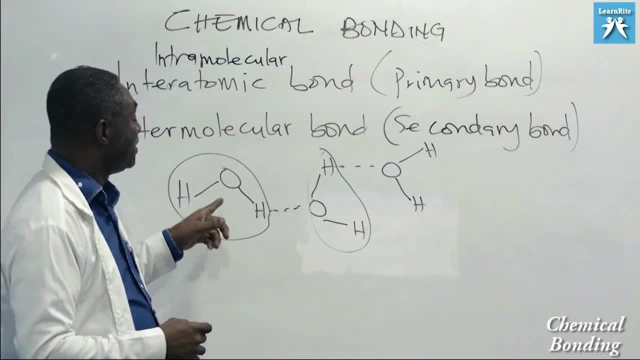 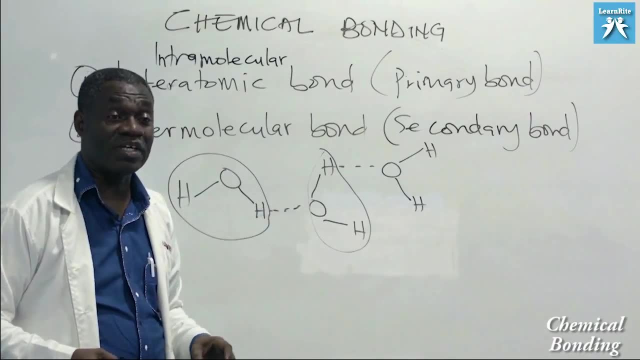 secondary bonds that are also very strong, because in some compounds or in some substances, the primary. you don't see a distinction between the primary and the secondary bond. they are the same type of bond, so they are equal, they become equal and you handle the bond between the primary and the secondary bond and you handle the bond between the primary. 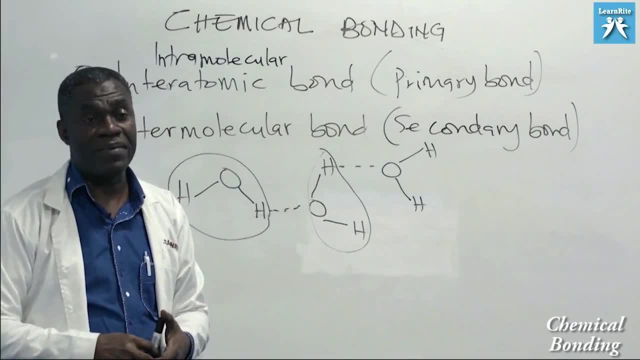 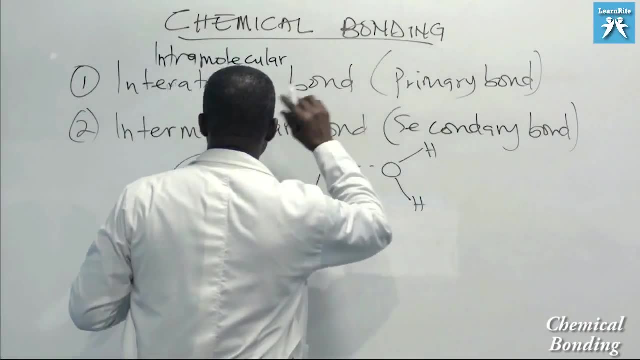 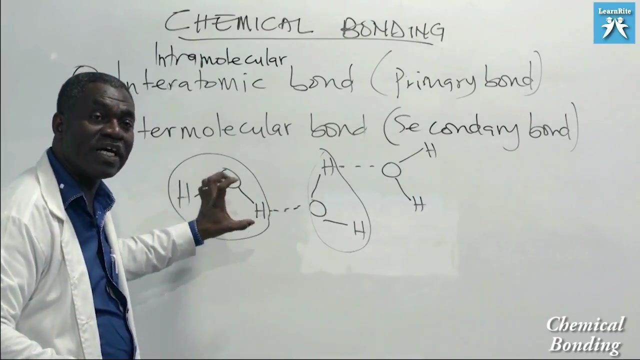 you get a secondary bond being very stronger or being stronger than a primary bond. so that is the basic illustration of what you mean: chemical bonding- two main types: inter-atomic or inter-molecular, that is, within one molecule, the forces of attraction that holds the atom together. 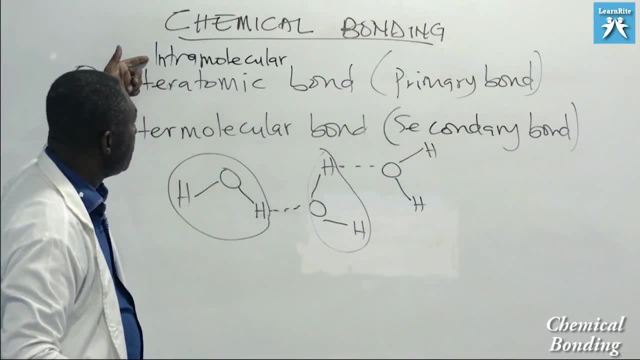 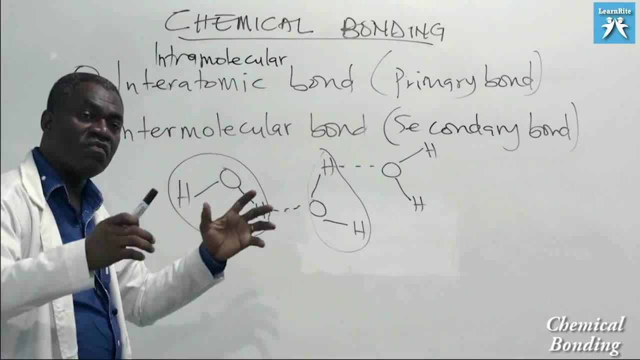 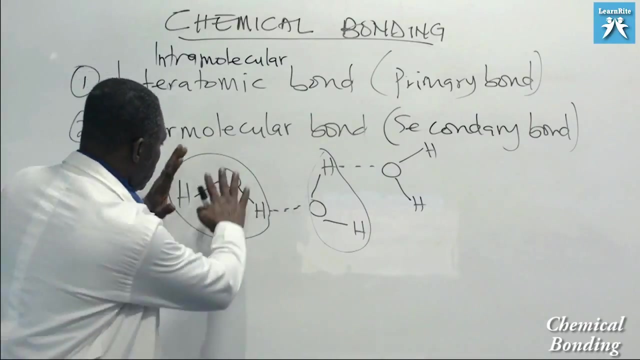 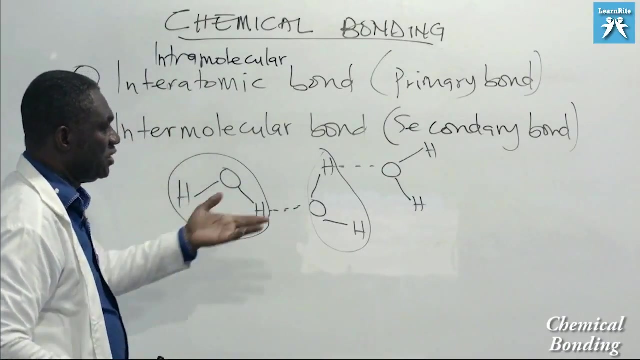 called a primary bond, other name is intramolecular bond, the main name being inter-atomic bond. then we have a second type of bond that holds the molecules of that substance together. that is inter-molecular. the inter means between what? between molecules, molecules, okay, and then the inter-atomic means that between atoms. so this is a secondary bond, that is primary bonding. 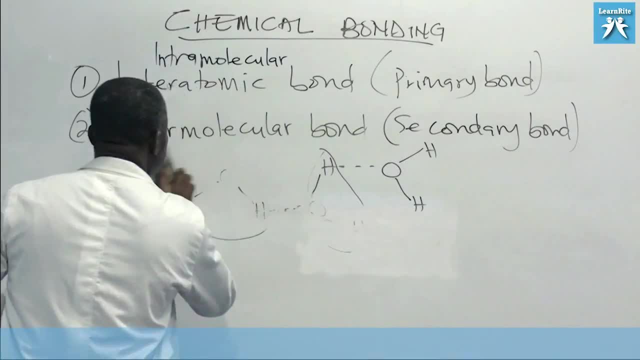 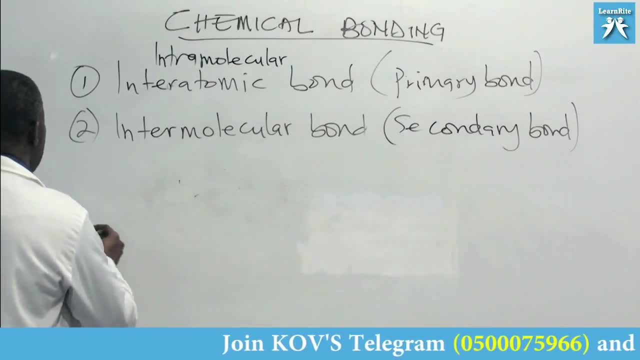 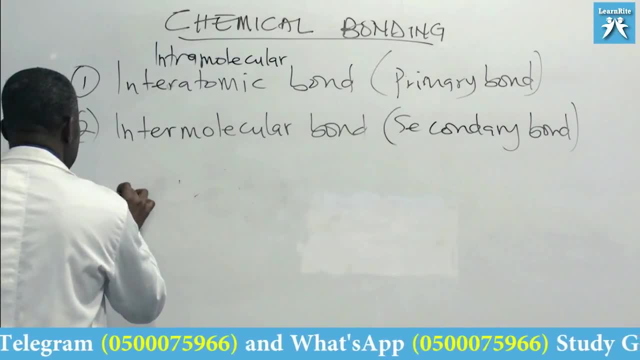 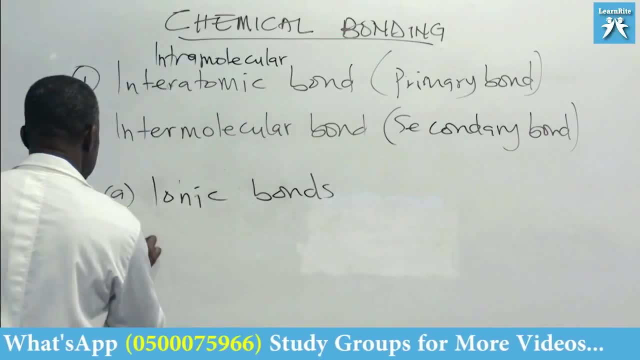 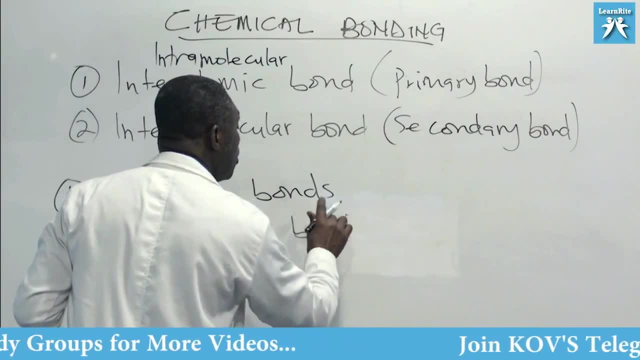 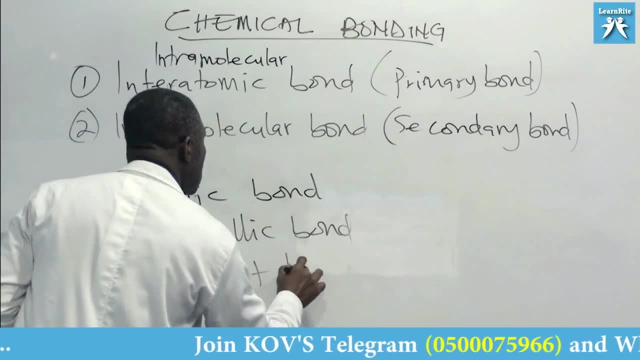 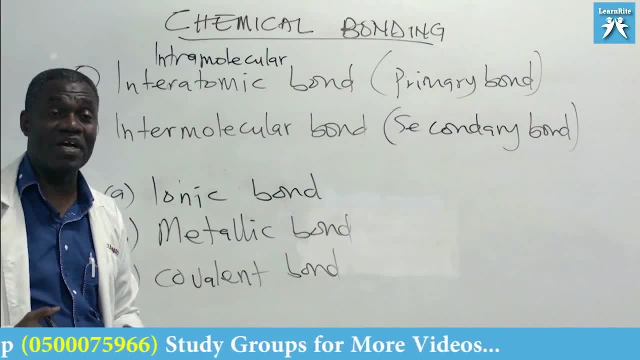 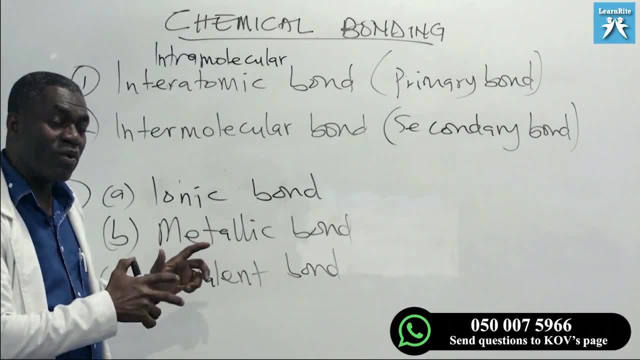 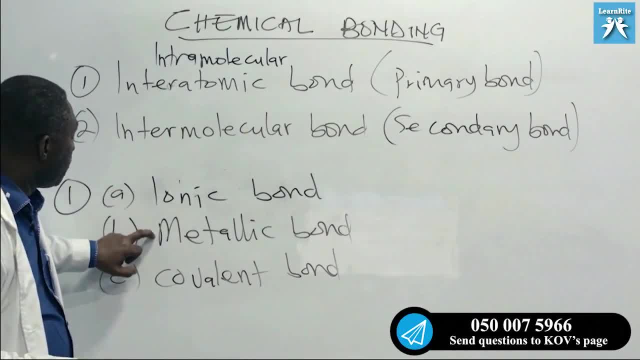 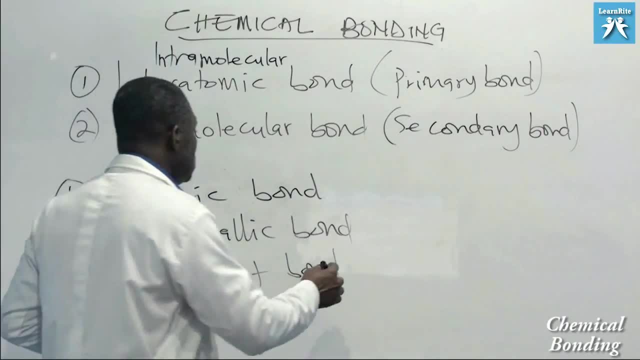 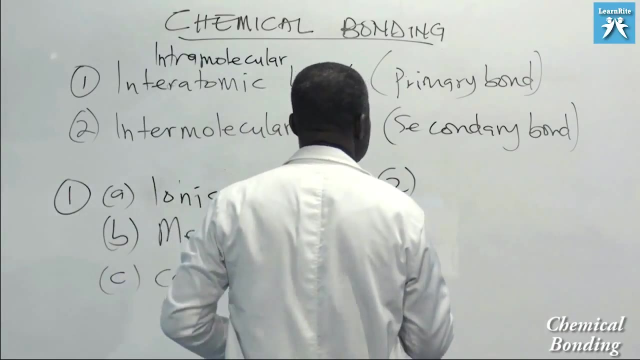 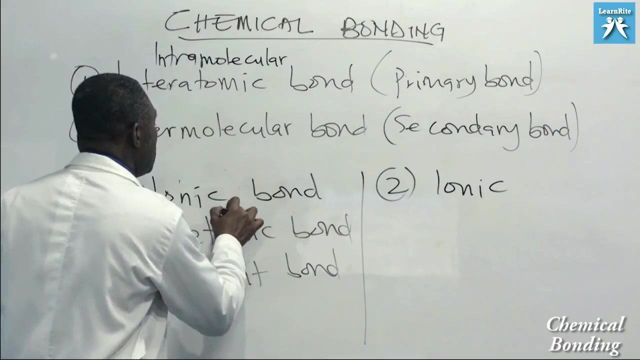 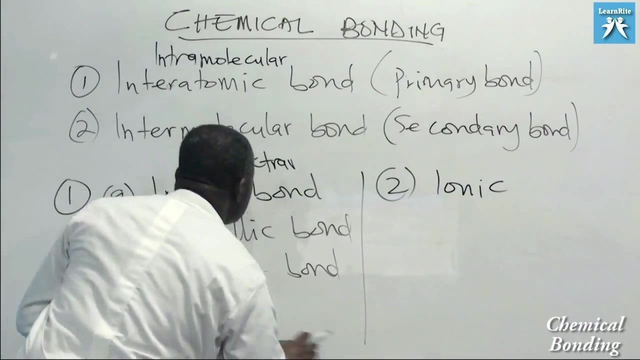 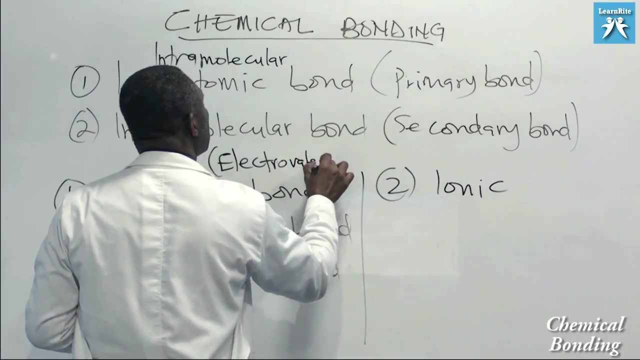 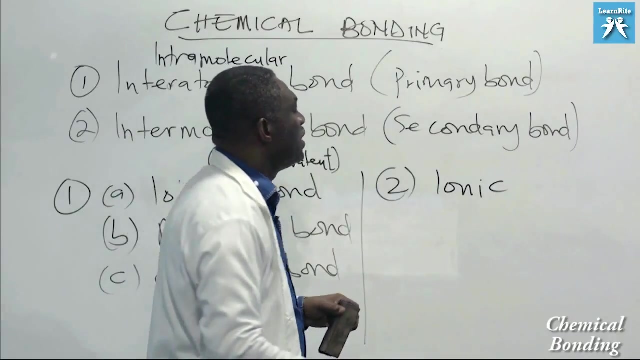 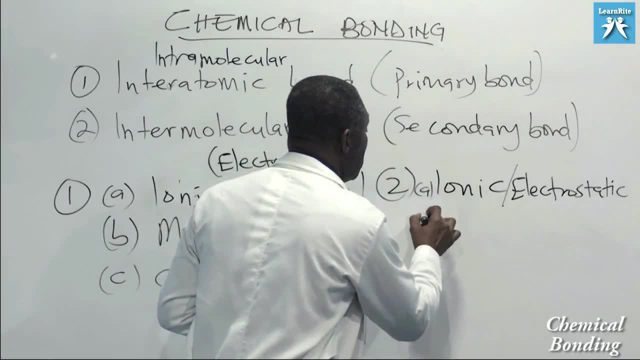 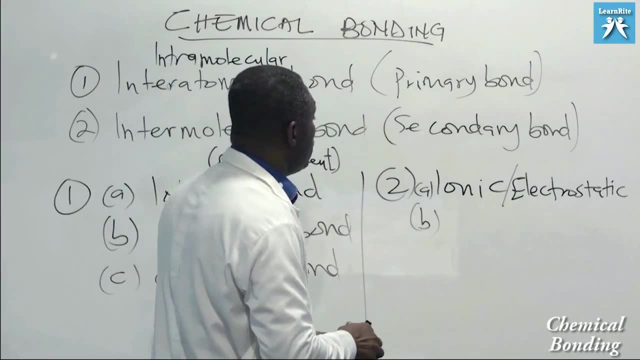 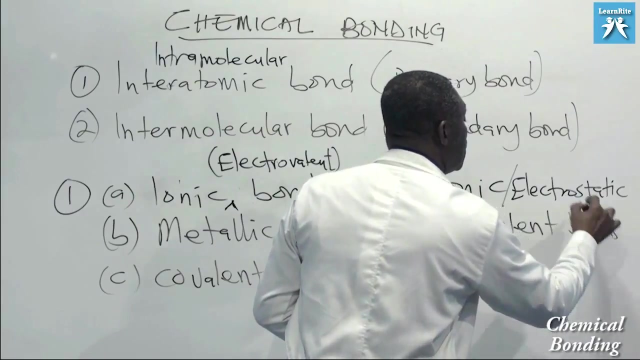 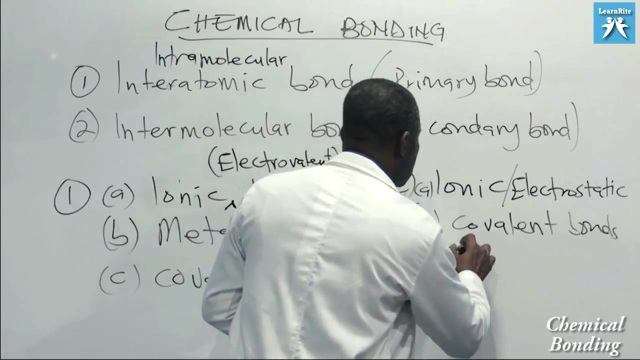 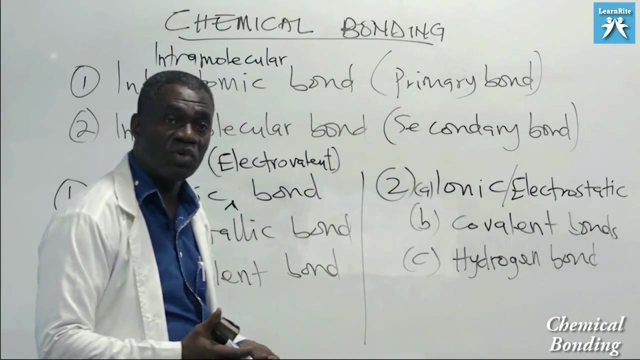 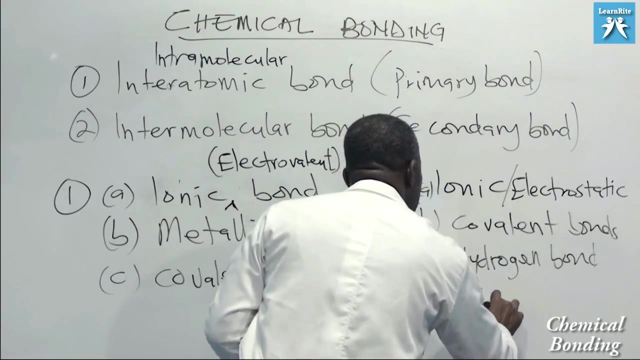 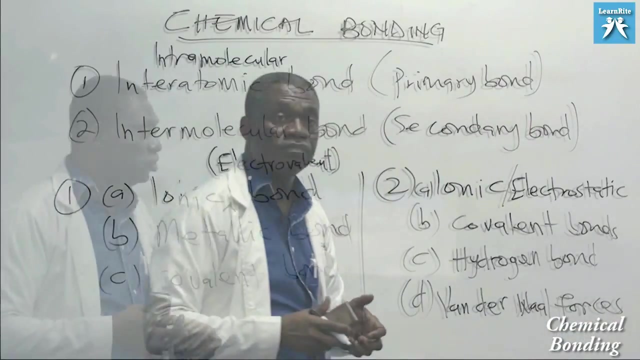 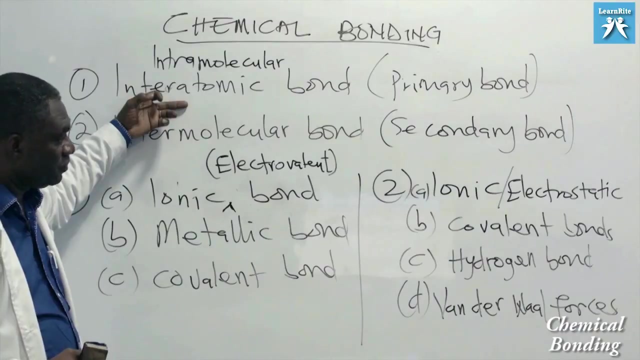 or a little violent bond, and then that is under the- uh listen, we also have equivalent, equivalent bonds. we also have covalent bomb being intermolecular, and then we have c hydrogen bond as an intermolecular bond and then one of our forces or private bonds. when we come to intermolecular bonds or forces, we still have inequality to. 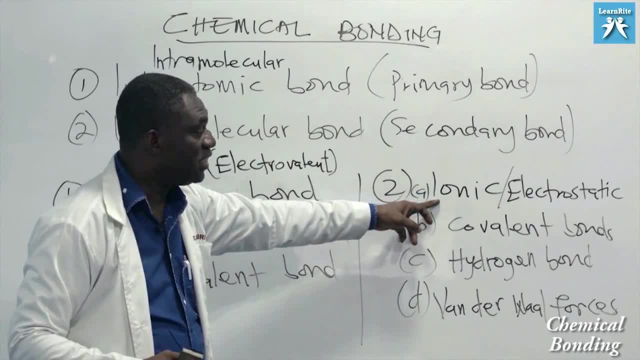 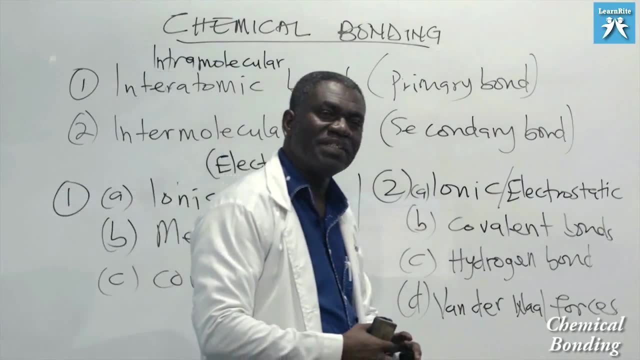 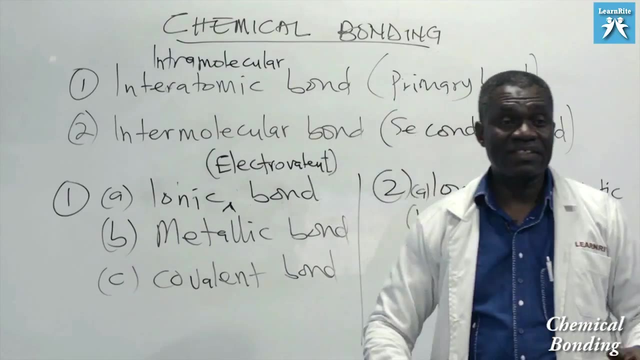 start it there. we still have covalent there, then we have hydrogen bonds and we have van der waal forces- now the very basis of life, as i've already mentioned, or the explanation to why substances exist the way they are. i'm coming back to the table to explain. what do you see here? 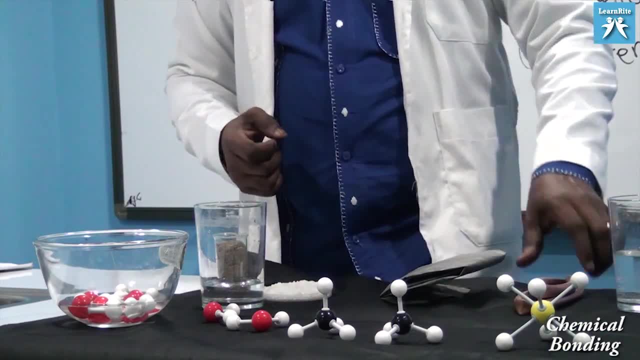 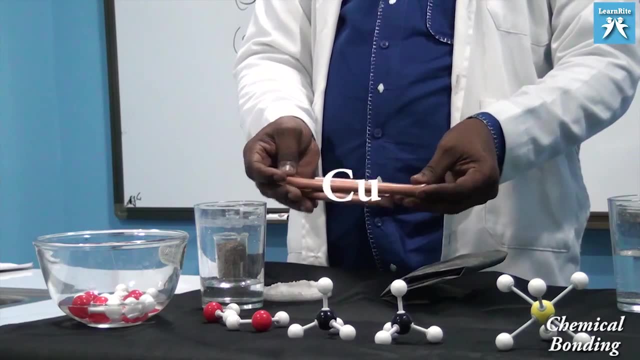 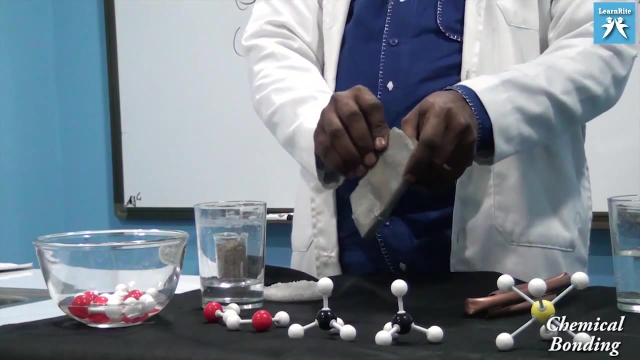 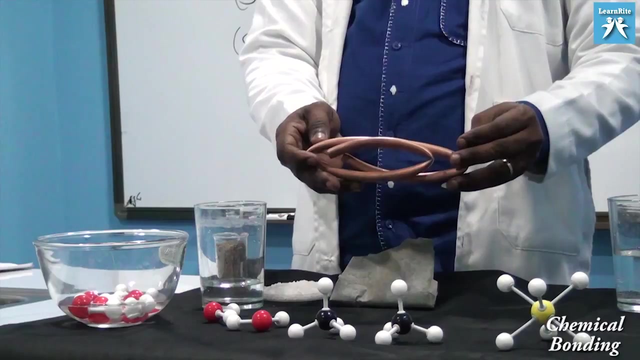 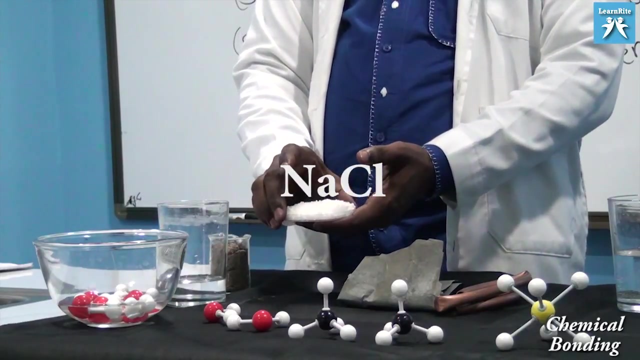 this is a very important thing for us to understand. i guess you know it. it is copper metal. this substance is aluminum metal. why is it that this aluminum metal is softer than the copper metal? this is sodium chloride, the ordinary salt. why is it not as hard as the metal? 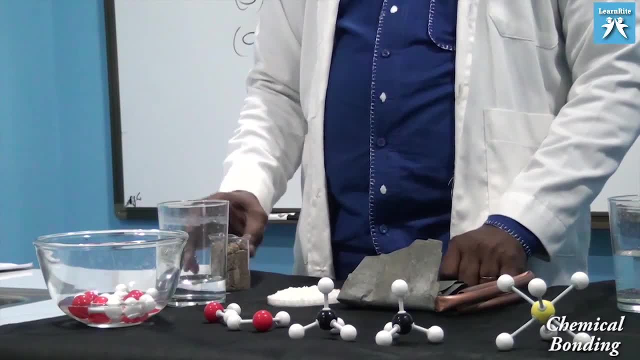 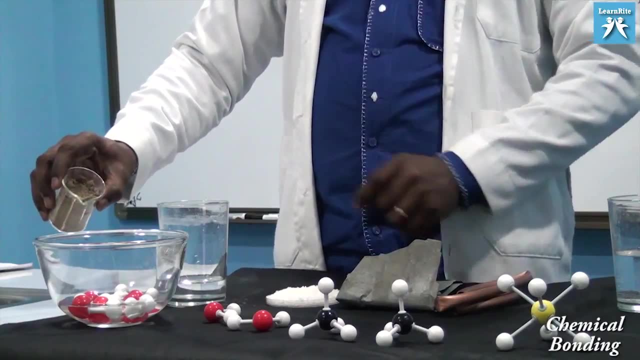 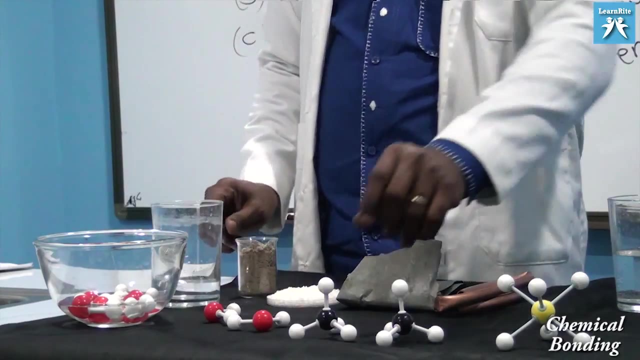 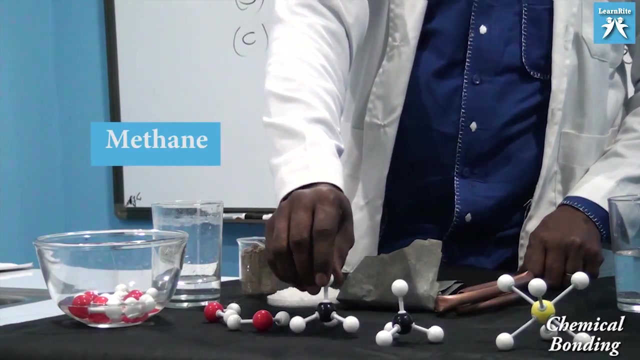 that i've illustrated first. this is the ordinary soil: f soil. why are they always in particles? if i begin to pour it here, you see that they pour in particles. why is it so? i've already illustrated the water. this is a molecule representing something called methane. okay, this is the shape of methane. 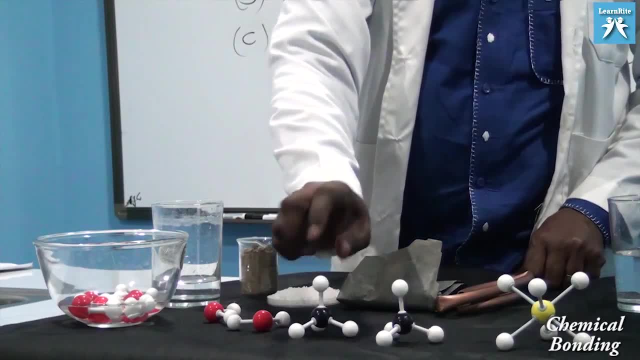 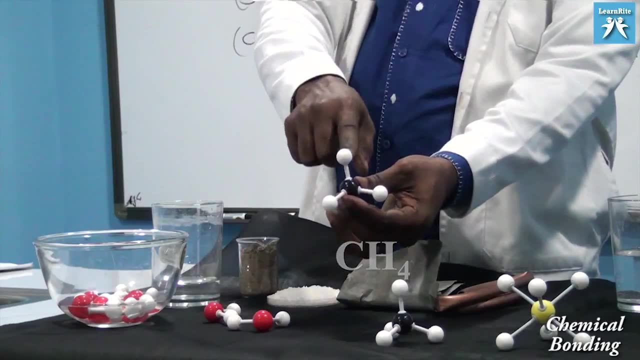 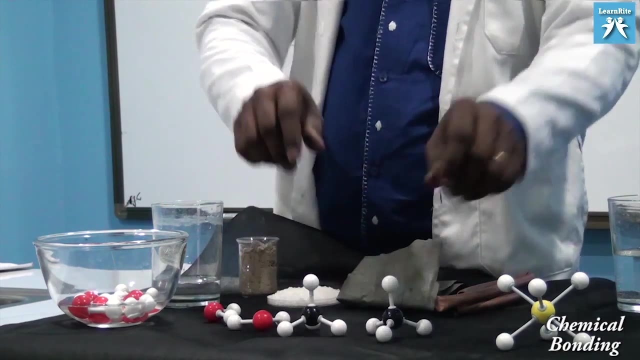 where we have carbon bonded to hydrogen, hydrogen, hydrogen and hydrogen, methane. the formula is ch4. or we could also say tetrachloromethane, where carbon is here and it's bonded to hydrogen, hydrogen, hydrogen, or it is going to chlorine, chlorine, chlorine, chlorine. that is the shape of it. all these that could also represent another molecule and, of course, 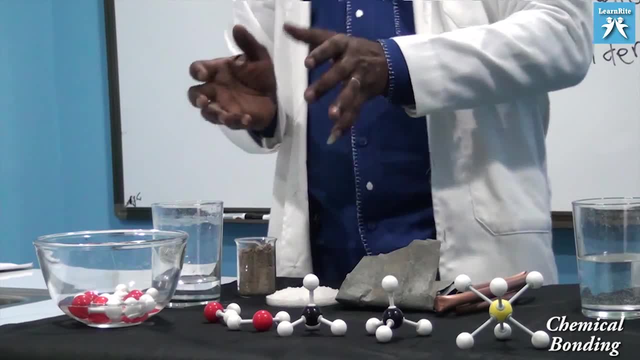 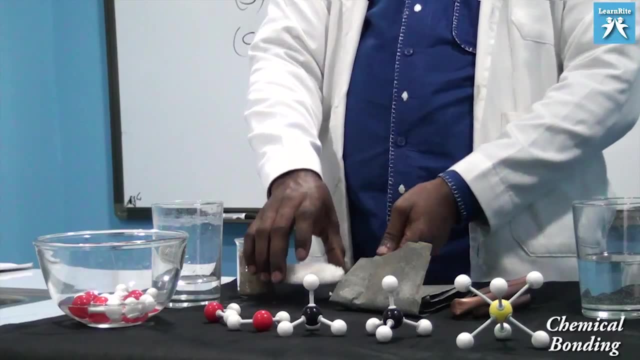 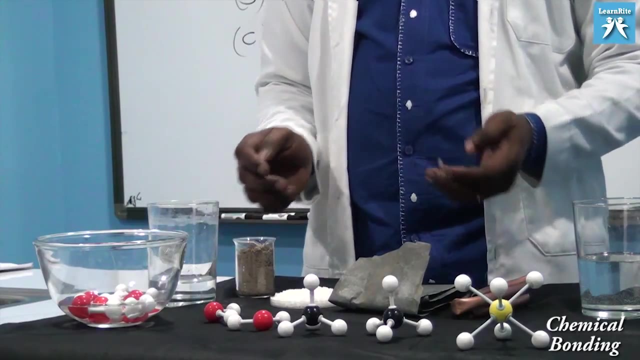 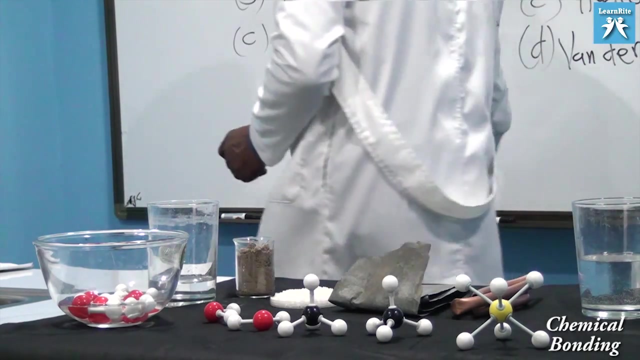 we have also our water here. why do they all exist in different states? the metals are kind of solid, the sodium chloride is also solid, the soil is solid, the water is liquid and unfortunately, because gases are not stable, i'm not able to illustrate a gas here. but let me say that, assuming i wrote, assuming i put oxygen gas there, i put nitrogen. 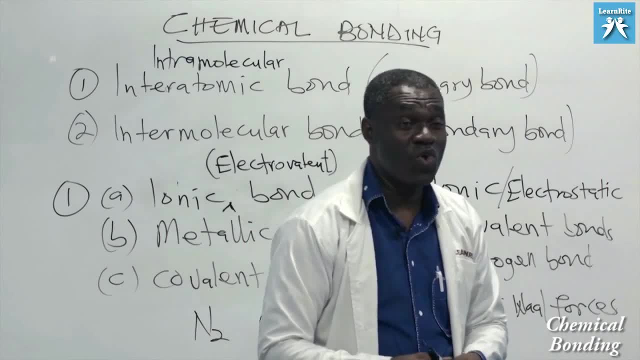 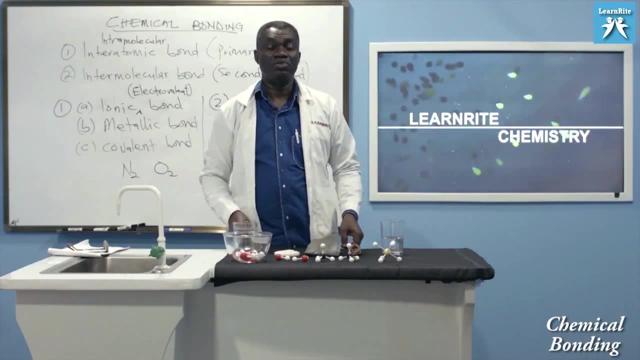 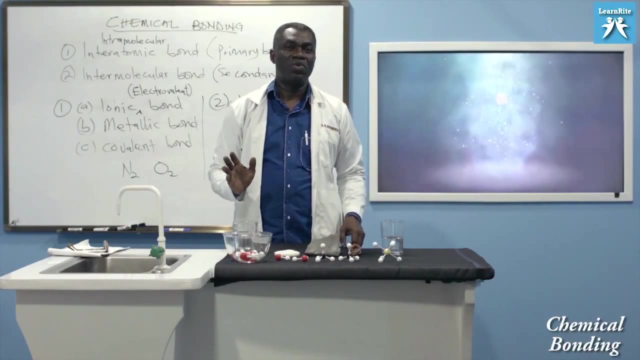 gas which i cannot see with my naked eye. but i know i'm breathing in the oxygen as i stand here and i'm teaching, i'm briefing in. you're also breathing in as you're sitting there. what are you breathing? you are breathing oxygen or there is air blowing around you? what is the? 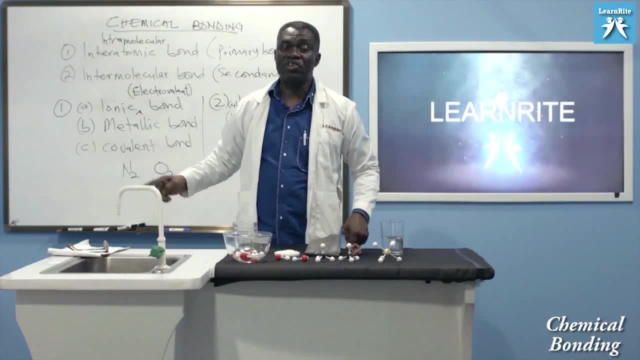 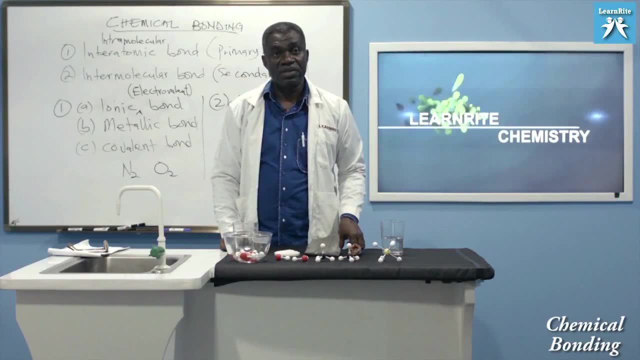 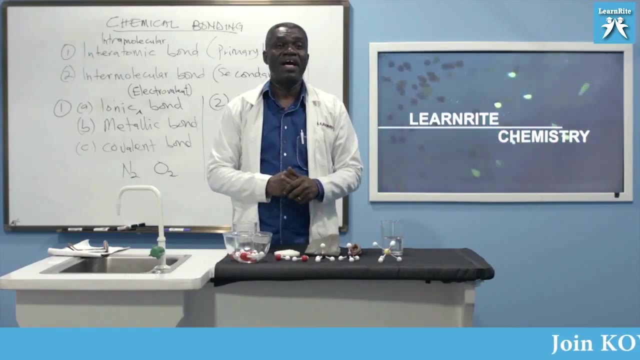 make of that air? that air contains oxygen gas, it contains nitrogen gas, it contains some carbon dioxide gas or carbon monoxide gas, gross types of gases. okay, and then, of course, in your kitchen you have the butane, propane condensed in a cylinder, as you call it gas for your cooking. they are all. 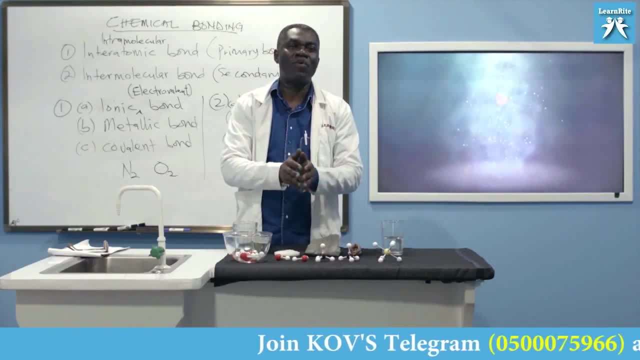 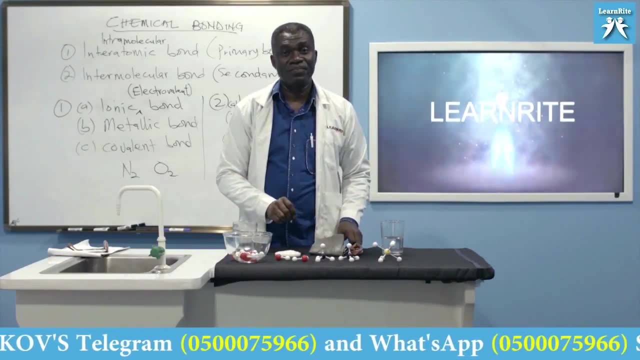 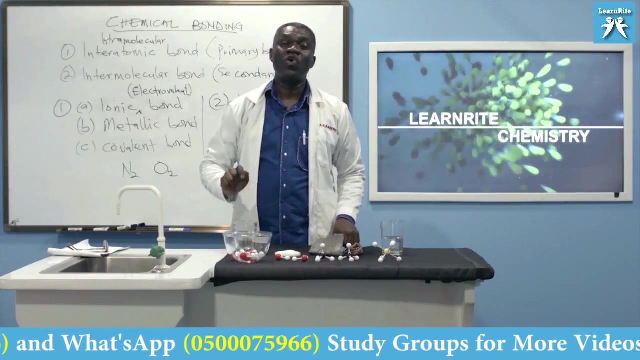 substances. why do they exist in the form of that gas? why is it that this exists as a solid and then sodium chloride also exists as solid? we have already said that attraction, force of attraction, is the basis of life, and so, depending on the strength of the attraction that exists between, 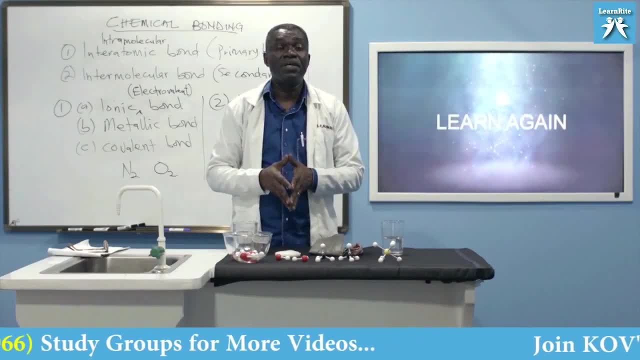 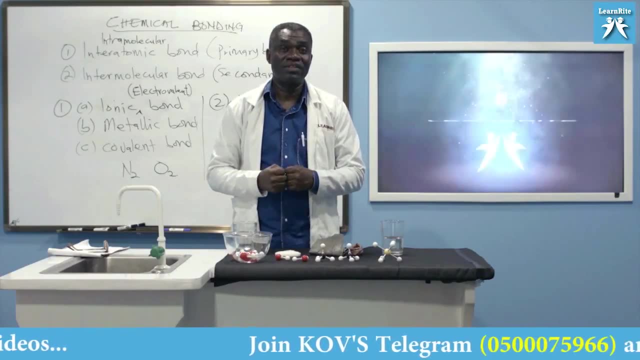 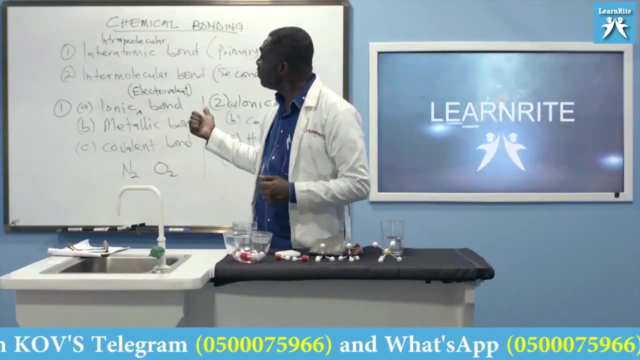 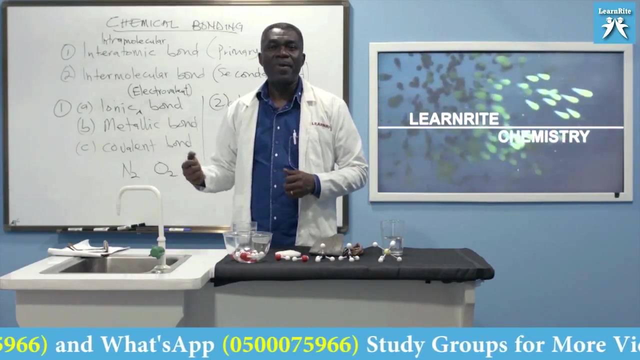 the molecules of the substance. the substance may either be a solid, may be a liquid or a gas. the force of attraction determine the state of any substance. if the force of attraction that is the intermolecular or the uh, the, that is the inter-atomic or the intermolecular, if 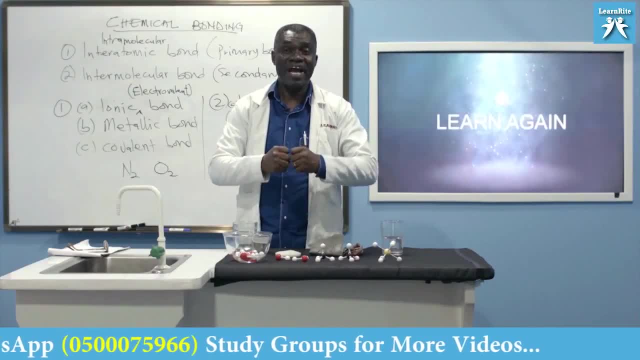 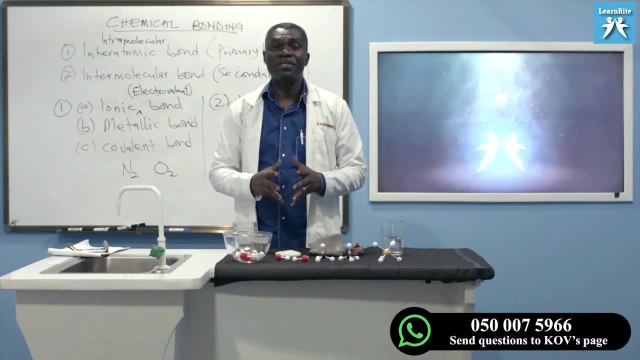 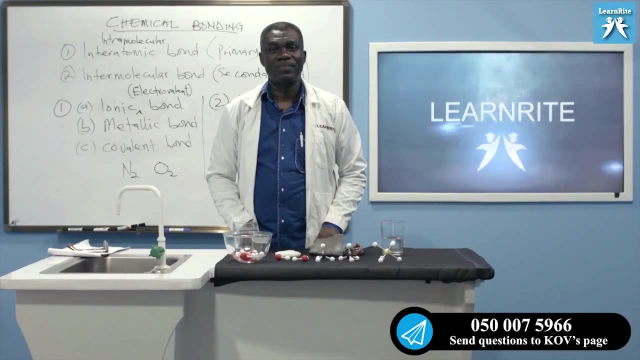 that force of attraction, which in chemistry we call bond, is high, then of course you exist as a solid, a hard solid. if it is weak, somehow you may exist as liquid, and it is very weak. you exist as what gas and some of the gases are. so, uh, some of the attraction, force of attraction.